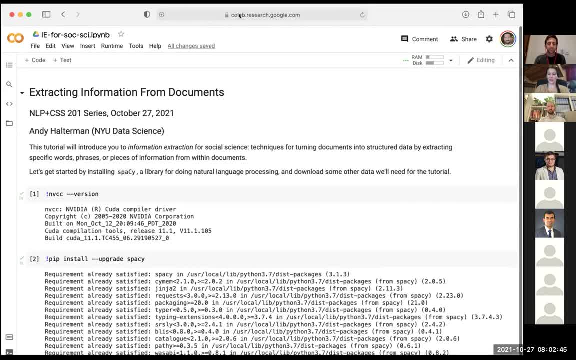 I'm Katie Keith. I'm currently a postdoctoral researcher at the Allen Institute for AI And I'll be faculty in the computer science and technology department And I'll be faculty in the science department at Williams College next year. I'm really excited to invite you to this tutorial series. I've been helping to organize it along with Ian And Ian if you want to introduce yourself. 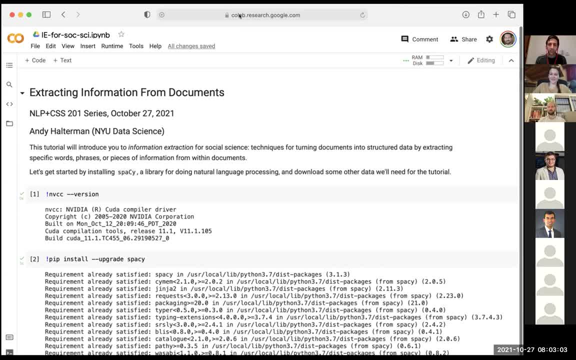 Yeah, hi, I'm Ian. Thanks everyone for coming. Some of you are repeat offenders. I appreciate that. I'm a postdoctoral fellow at University of Michigan in computer science And, yeah, like Katie said, happy to be here and co-organizing this. 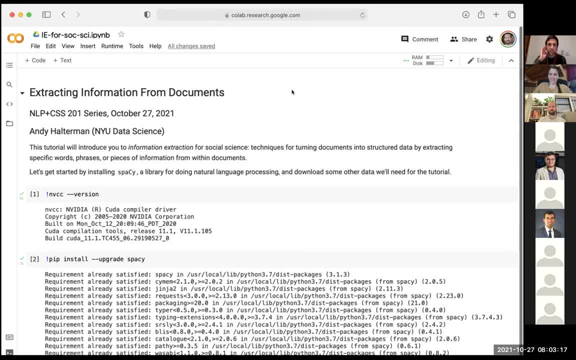 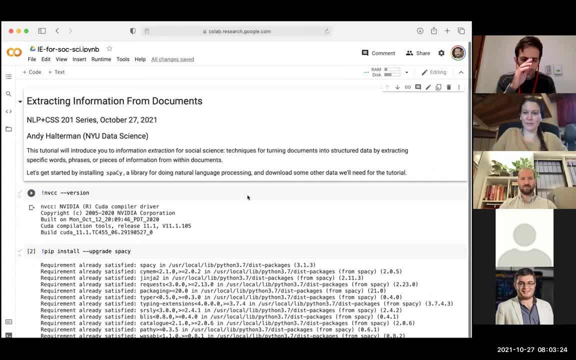 So with that, I guess, Katie, we're going to turn it over to Andy, right? Yep, All right, cool. Today's facilitator is Andy Halterman, who is a postdoctoral fellow at NYU, And he is going to be leading a really awesome tutorial about information extraction. So, Andy, why don't you take it away? 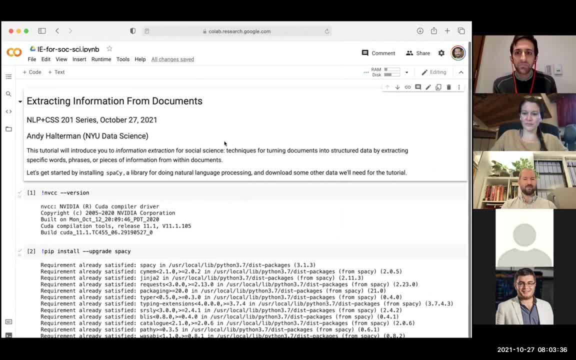 Yeah, great, Yeah. so I'm Andy. I'm a fellow at NYU in data science this year, but I'm actually a political scientist. So I just finished my PhD in political science And then next year I'll be at Michigan State as a professor in the political science department there. 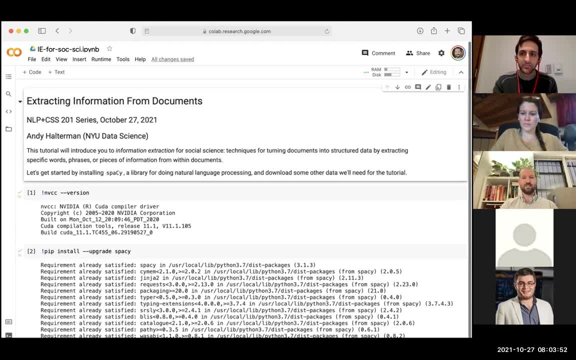 Just a sort of a few notes as we get started. I just sent a link out in the chat to this notebook, So feel free to make a copy of it and follow along. There are a few interactive demo exercise type things later on. that, I think, will be more fun if you're if you're doing it along with all of us. 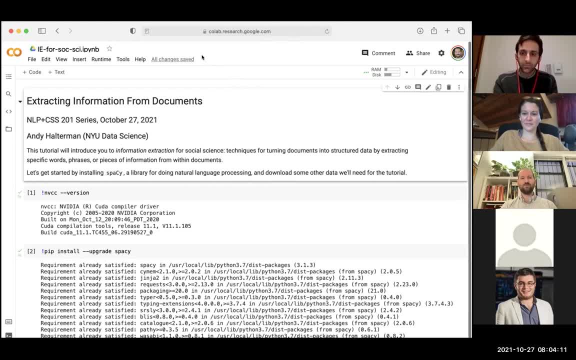 If you have any questions or anything is unclear, it would be. I would really appreciate you bringing them up, because if if you're confused, then almost certainly someone else will be confused. So I think it's probably easiest if you have any questions. 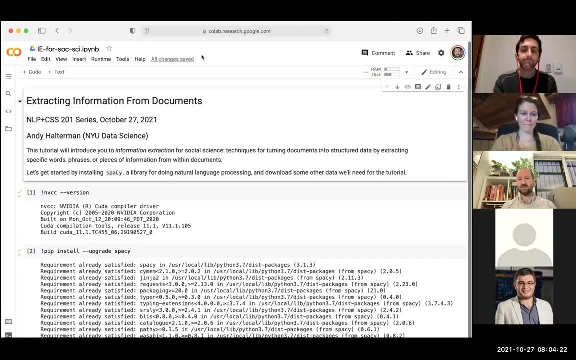 So I think it's probably easiest if you have any questions. So I think it's probably easiest if you have any questions. So I think it's probably easiest if you just put it in the chat And I think Katie and Ian will be watching the chat as much as they can and then they can. they can stop and interrupt me. 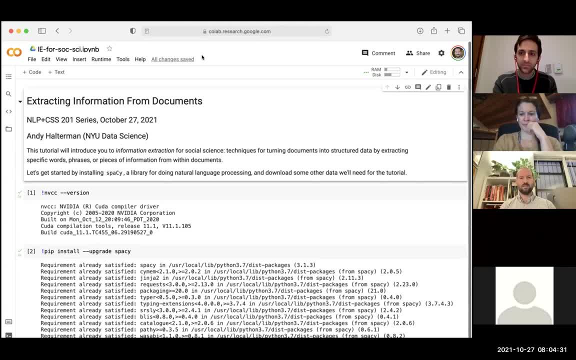 But we think we have a. we have a nice sized group, So this doesn't have to be a sort of YouTube I speak to people thing. This can be a you stop and you have questions and we'll have some discussions. So I think maybe, as new people join, we'll have to resend the link to them in the chat. I don't think they see the chat history. 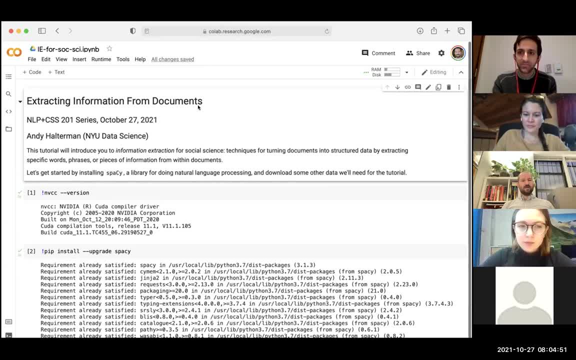 Great Yeah, so So the the thing I'm going to talk about today is is what a lot of my research is on, which is: how do we extract information from within documents to answer questions in in social science? We'll talk a little bit more about what it means to extract information from documents or to turn documents into structured data later. 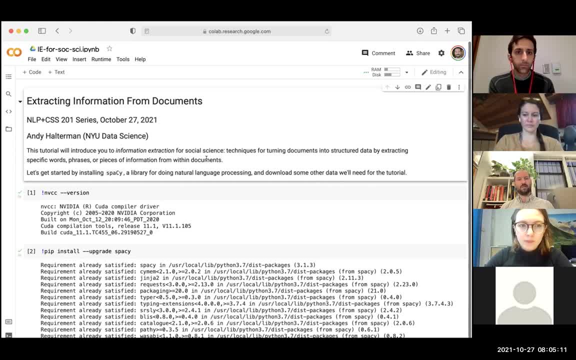 But first I wanted to give people a moment to to make a copy of this notebook and run the first few cells. so we're using them. An LP library here called spacey, and spacey depends on a few large model objects that take a little while to download. so it will take about a couple minutes to download those models and then in a moment it's going to take about maybe five minutes to process a large 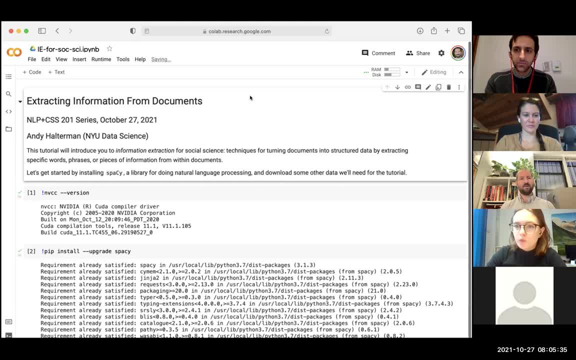 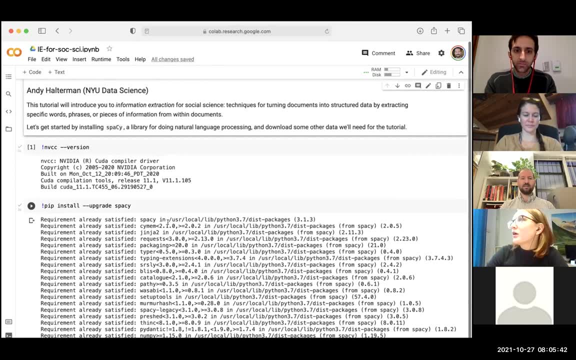 collection of documents that we're using. So, as I'm talking, go ahead, make a copy so you can edit it and then start running these cells. Yeah, so we're going to get started by installing spacey, which is a library for doing natural language processing in Python, and then we'll download some data we need for the tutorial. 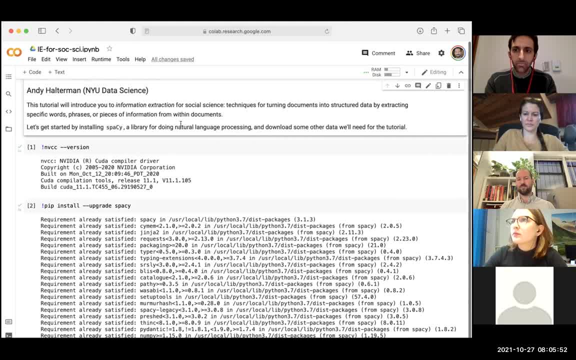 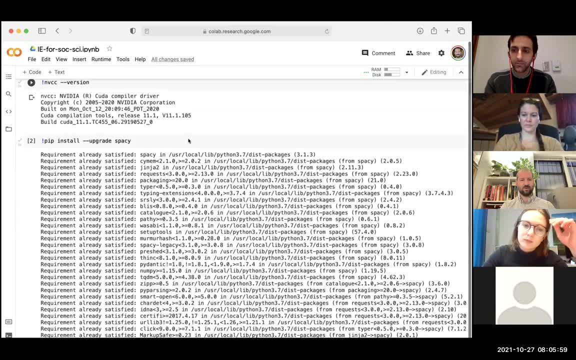 I think I think the assumption for everyone in the tutorial series is that you're familiar with Python. But again, if there's any sort of confusing things I'm doing in the code, please stop, because I'm sure if you have the question, other people have the same. 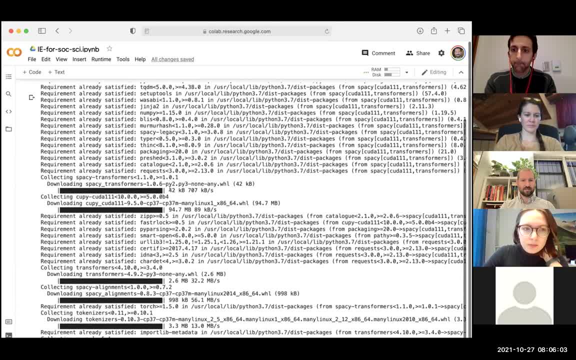 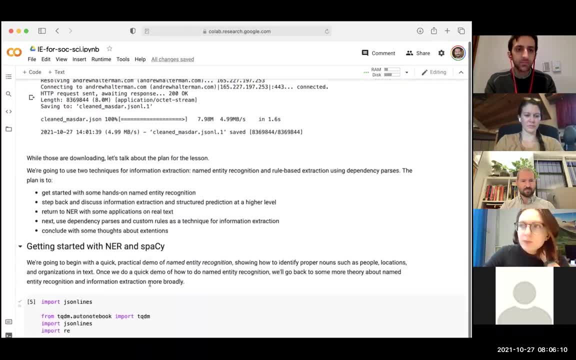 question. Okay, so I'm just going to scroll past the installation here And the download Should be done, running for me. Okay, so, while those are downloading, I just wanted to briefly go over what the plan for the lesson is today. 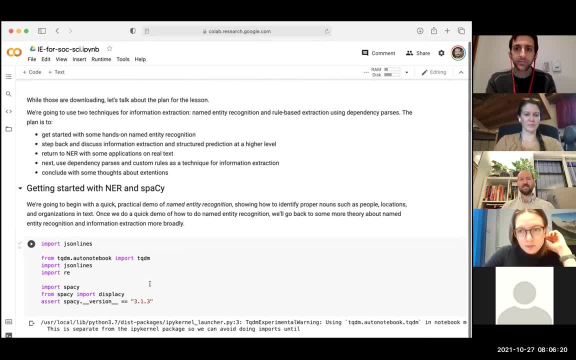 So we're gonna talk about two specific techniques for information extraction: named entity recognition and rule based extraction using dependency parses. So those are the two techniques are going to cover And the plan is we're just launching to doing some- some any are right at the beginning so we can see what it looks like to to extract information from a document. 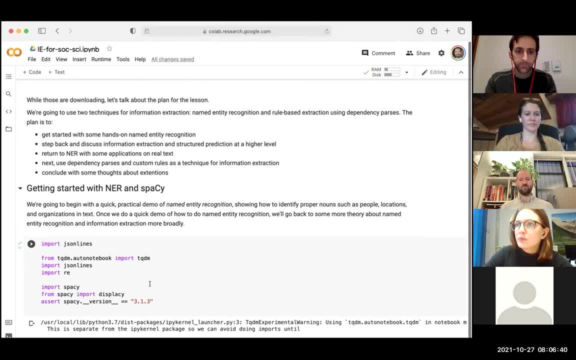 Then I want to step back and talk about things from a more theoretical perspective. so what does it mean to do information extraction and what is structured prediction? Then we're going to go back to the NAR and do some applications and exercises on real text. 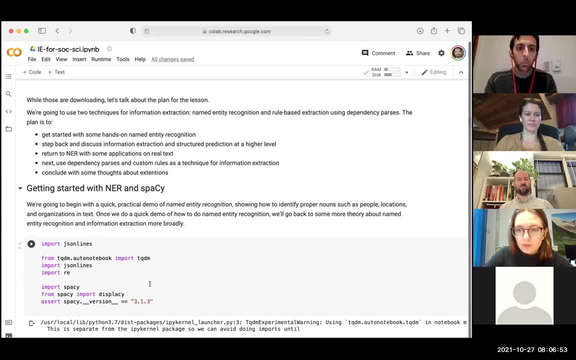 Then we'll do the second technique, which is using dependency parses, which will go into more detail about and writing custom rules as a way of extracting information from documents, And then, finally, there'll be some sort of extensions and other other interesting things that you can do at the very end that will 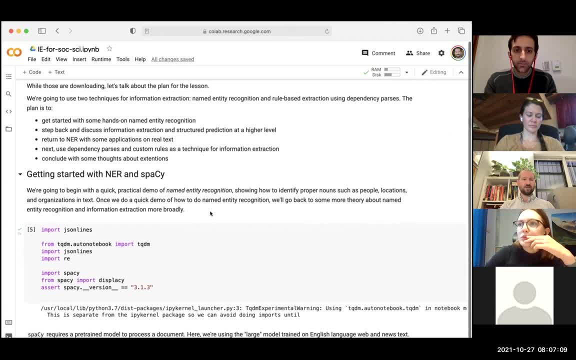 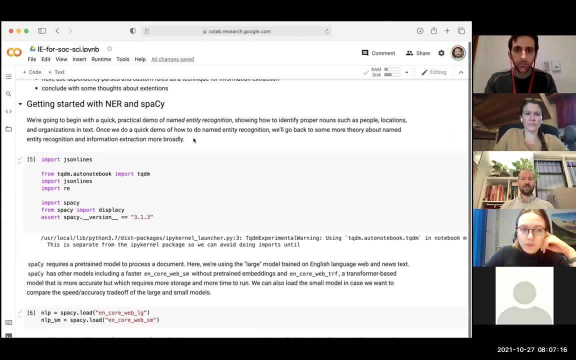 Do more or less of time permitting. Okay, so getting started with with any are and and spacey. So essentially what any are is is identifying proper nouns in a piece of text, so identifying things like people, locations, organizations or some more obscure things that are sort of stretch. the definition of named entities, like mentions of currency or mentions of numbers. 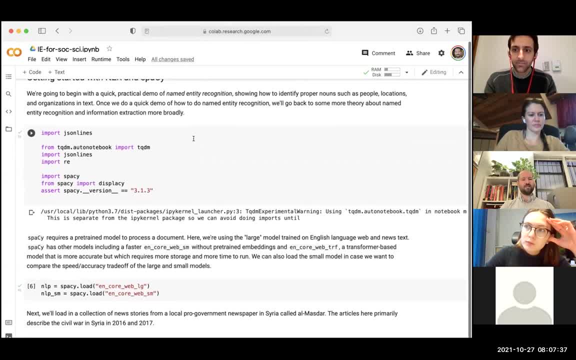 And The way that we're going to do that is using a Python library called spacey, and spacey does a lot of different NLP techniques, And that's what we're going to use to do both of the named entity and the dependency parsing. 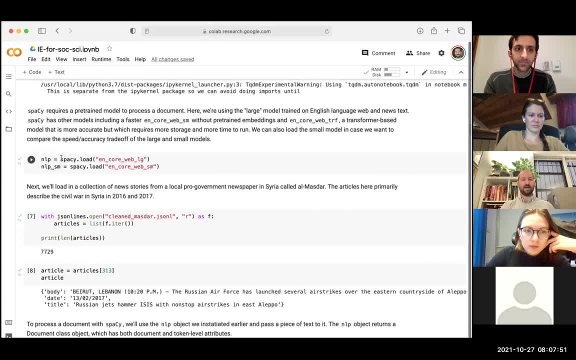 So, in order to work So spacey is a machine learning as a machine learning back end to it And to to use it, we're going to load These two models that it can use, so there's a different size, models that have trade offs between speed and accuracy. 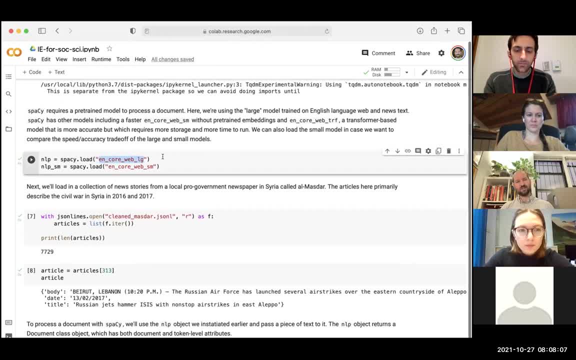 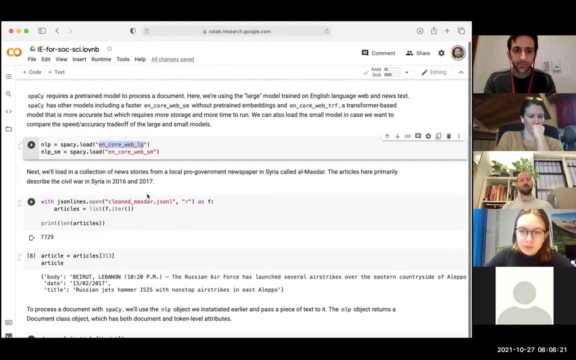 So we're going to be using the large model, which is actually not the, not the biggest model, but is sort of a nice balance of speed and accuracy. Then we're going to load in some some new stories and this is what we're going to be working with for the rest of the tutorial. So these are articles that I scraped for for a project. 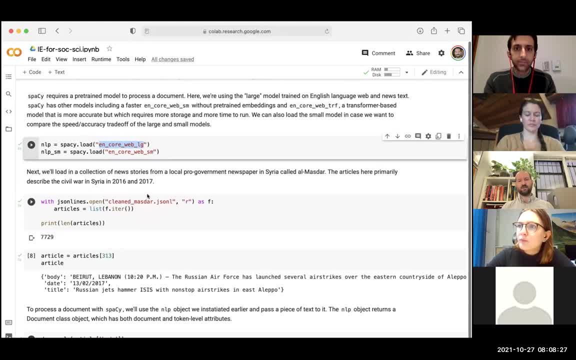 Some of the research that I do on violence against civilians in Syria and in this case it's a- it's a pro regime English language newspaper called all master. So it's about Seven or 8000 articles published in 2016 and 2017.. They're all English language and they mostly focus on on the fighting in Syria. 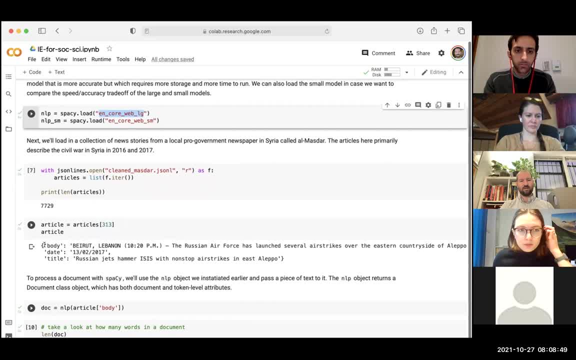 Just to show you what these articles look like, if we just print out one of the articles that has three keys here in the dictionary body, which is the main, the main piece of text, a date and a title. and we're really only going to be working with, with the body. 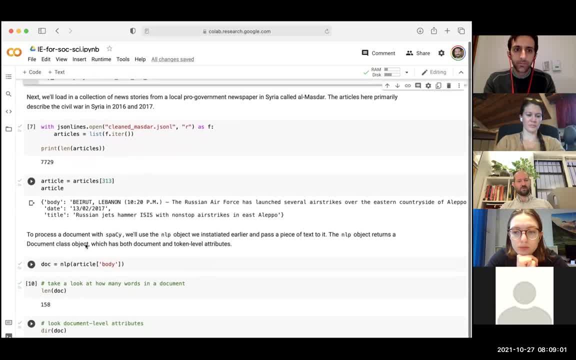 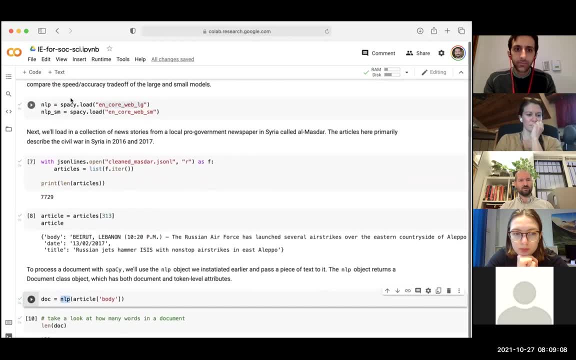 here. So to put an article or put a piece of text through spacey, We're going to do that is by calling this NLP object that we instantiated earlier. So just to review this: NLP objects we create by loading a model and then we can use this NLP model to process documents. 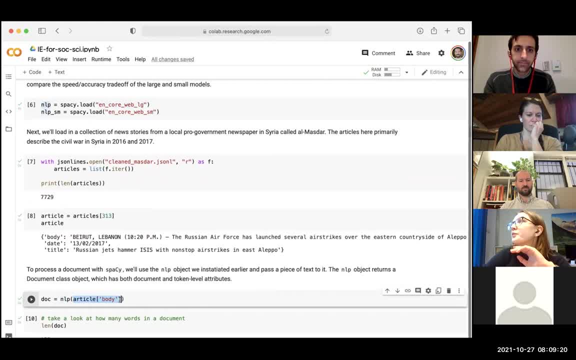 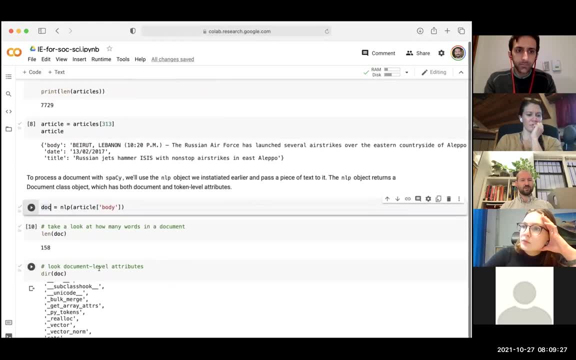 So we're going to take this NLP object and put the body of the article through it and we get a document out. So just to sort of start to familiar ourselves with what this looks like. So the way that spacey represents a document is it will split into tokens, which is a very familiar task for anyone who's who's worked with text. 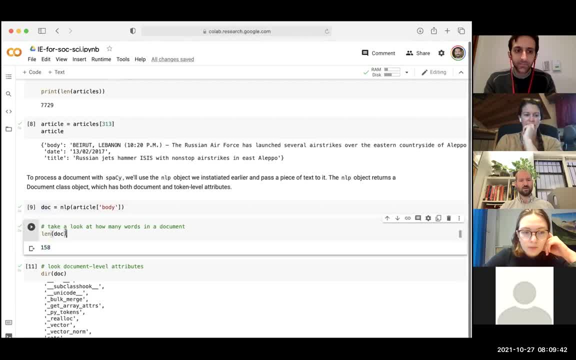 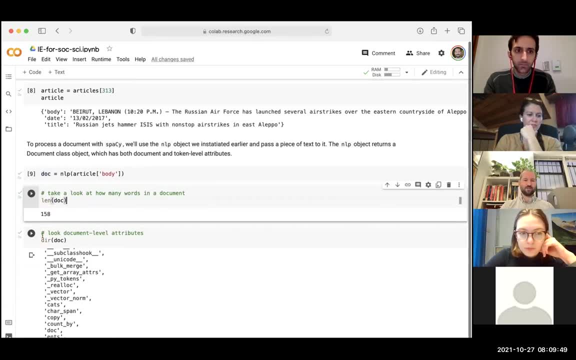 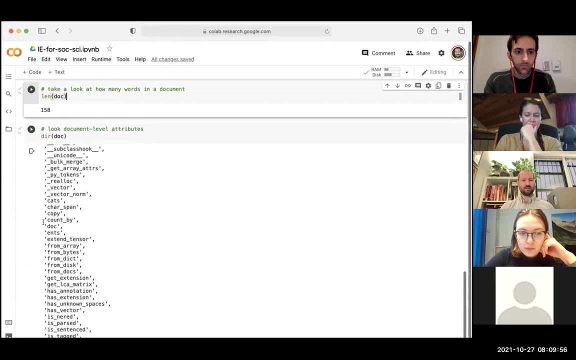 So split into tokens- In this case that is 158 tokens or words in the document- And then it provides both document level attributes and token level attributes. So we can just use the the dir function here and see what it gives us at the document level, right so? 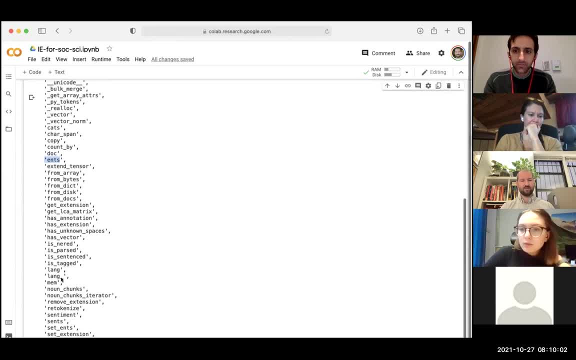 It's giving us entities, which will come back to later, but all sorts of other stuff like it'll provide noun chunks or tell us what language it is, it will tell us if it's been parsed already or not, And so all of these are things that we can we can use for other applications, but we'll really be focusing here on the, the entities. 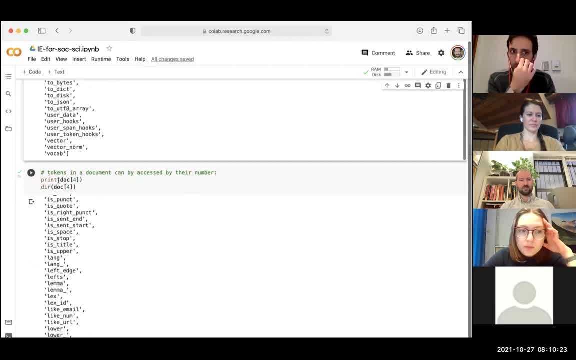 So in spacey tokens can be accessed by their number. so here in this document object we can access the fourth token. So in spacey tokens can be accessed by their number. so here in this document object we can access the fourth token. 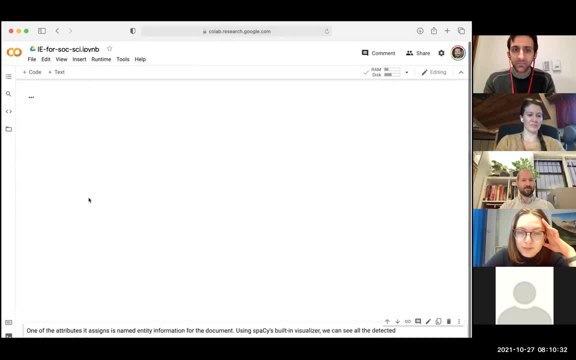 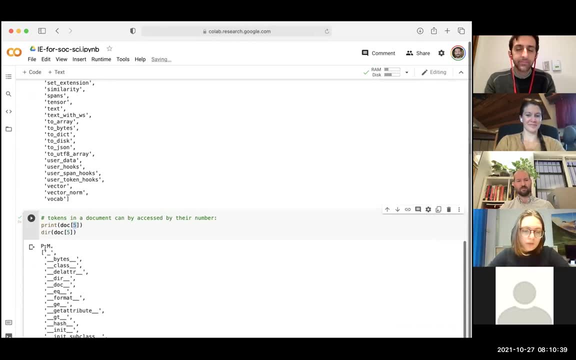 So in spacey tokens can be accessed by their number. so here in this document object we can access the fourth token, which is kind of a boring token actually. So here the fifth token is the term pm, so it's part of a time. and then this token also has attributes like: has it been parsed? 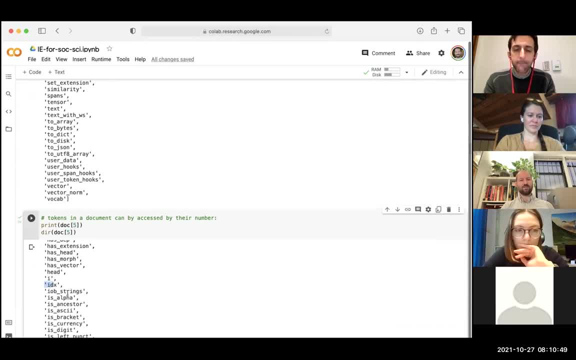 What, what number is it in the document, what characters in the document and so on. So there's a lot to explore here that we're not going to go into, but this is sort of what space is providing to us at the, at the token level. 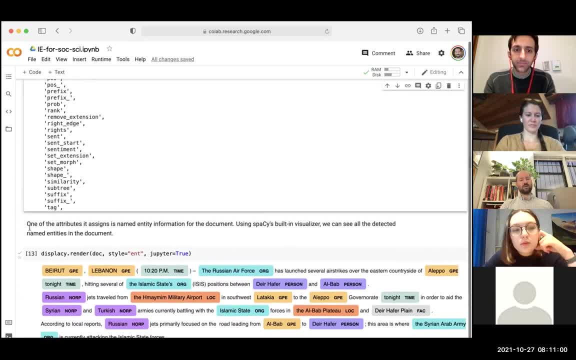 And so this is kind of a boring token, actually. Okay, and so, as I mentioned before, one of the attributes that it assigns at the document level is named entities, so we're going to use spaCy's built-in visualizer for entities. 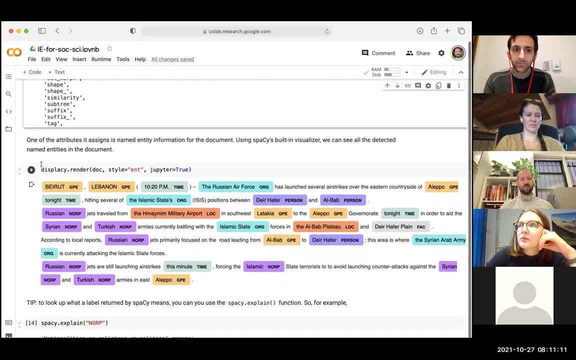 and see what entities are detected in this document, and we can use this displayC function that spaCy provides. We can say: render this document showing us entities, and this is a Jupyter notebook, so make sure that you do that correctly. 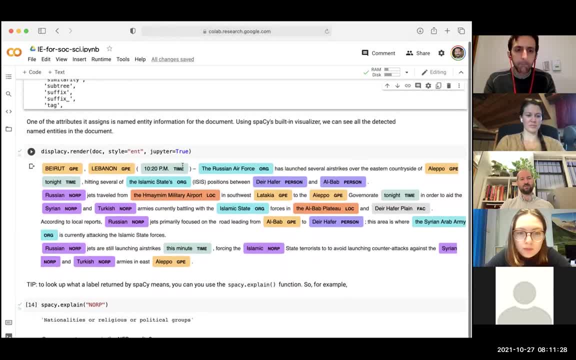 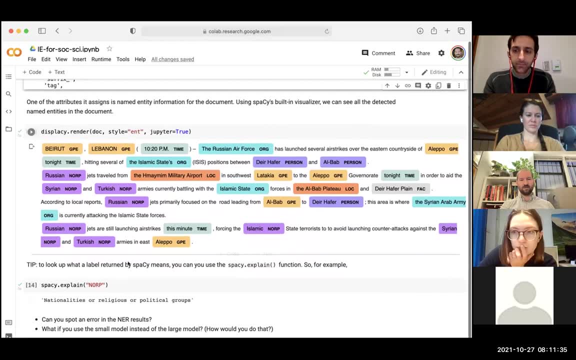 So, as you can see, it's printing out the article and then giving us labels for different named entities, and a nice function that spaCy provides is this explain function, so we can give it a tag that we don't know, like what is NORP, and it will tell us what that tag. 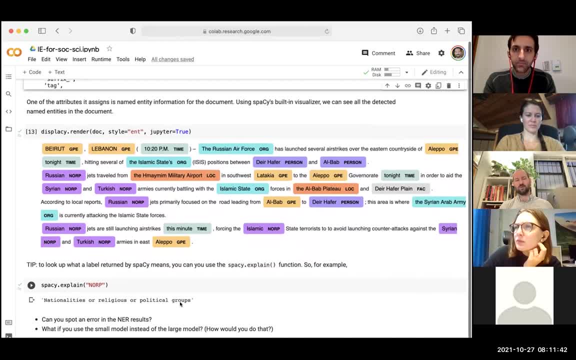 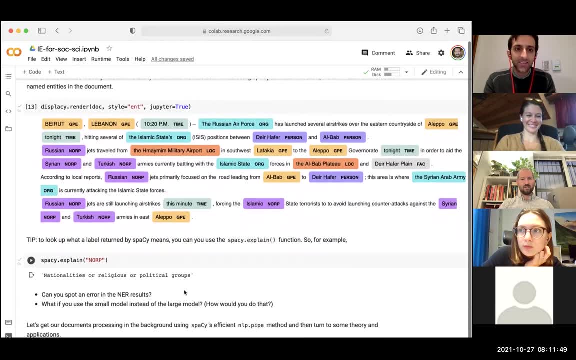 means, and you can use that for other things, like the dependency parses we'll use later, or parts of speech tag, if you don't have them all memorized, which I don't Okay. so at this point I wanted to stop and look at the document and think about you. 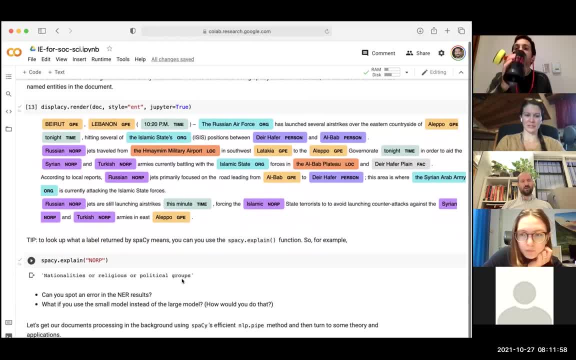 know, is there one thing that's important with all of this, which is: do you see any errors in this document And if, like if you don't know what GPE is, you can look that up too. I see something in the oh gauged the link. okay. 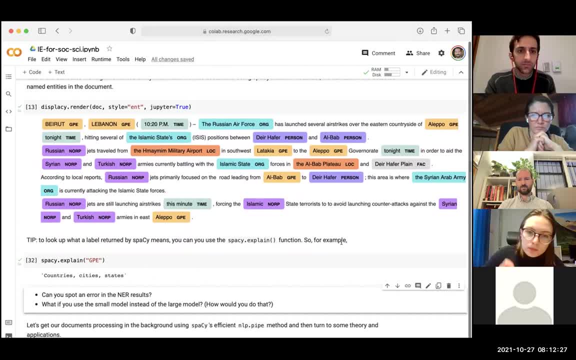 Okay, Yeah. so anyone spot a? anyone spot an error? here We have in the chat a couple of answers. I don't know if you want me to read them out loud or just let them flow in. Sure, I can read: yeah, so, yeah. so all Bob is not a person, that's right. so here. 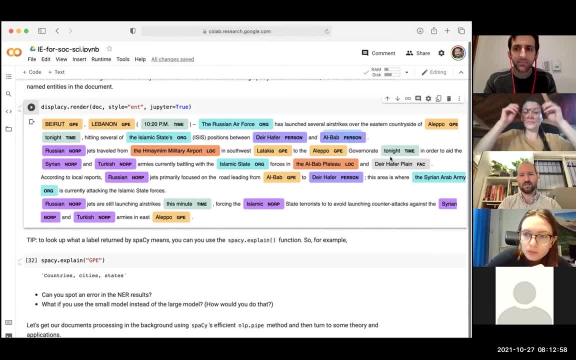 this, this mention at the end of this sentence: this is actually a town, so it should have the GPE label. and then Connor has a, has a very insightful social science point, which is the Islamic State has sort of an. there's some ambiguity about when it's an organization. 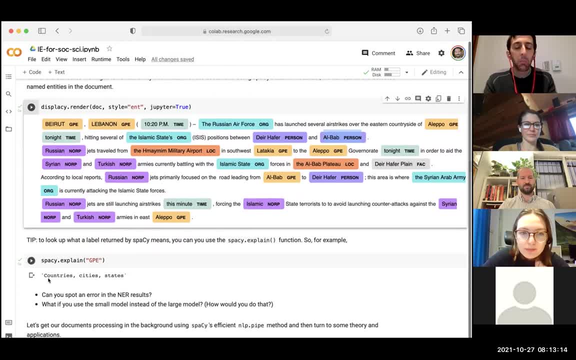 and when it might be called a GPE, which is the term used for geopolitical entities like countries. Yeah, those are both, both great points. one, one sort of social science and one sort of computer science. So you know the, the, the definition that's used by. you know the people who created. 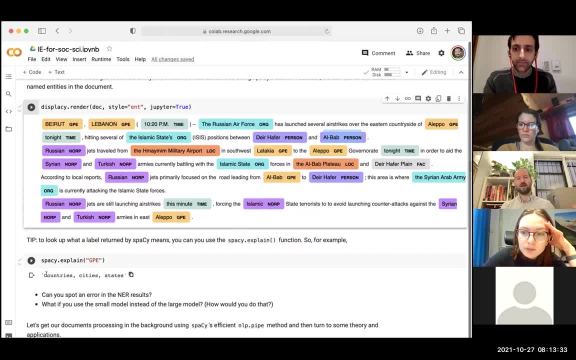 the training data for this 10 years ago might not match what we as social scientists actually want And then second the. the training data can just be wrong in or the sorry the model trained on. the training data can be wrong for ways that flow from the nature of the. 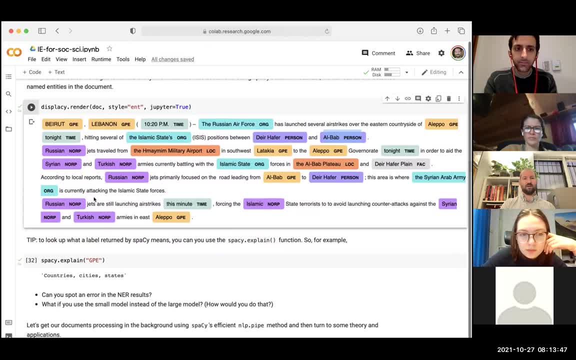 training data. So in this case, in my research using this on on text that includes a lot of Arabic place names, it performs quite badly because it's mostly trained on things like the Wall Street Journal or European and American news stories that that tend to not mention at. 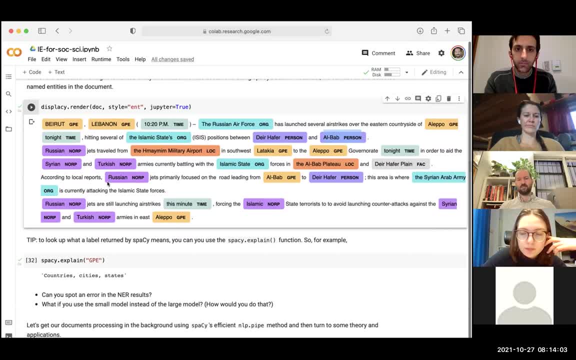 least in the 1990s, when a lot of this data was collected, didn't mention a lot of Arabic place names, Right. So there, there are consistent biases in how well this performs. So if you give it, if you give an article from Reuters about American politics, it'll. 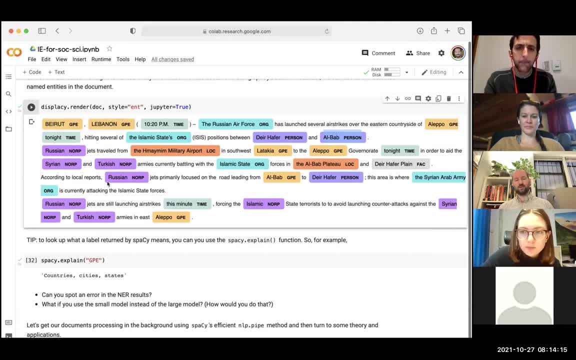 do quite well, And if you give it a local Syrian paper, it's going to start making more errors, Right? So it's always important to keep in mind what it's trained on, and the further you get from that, presumably the worst it will be. 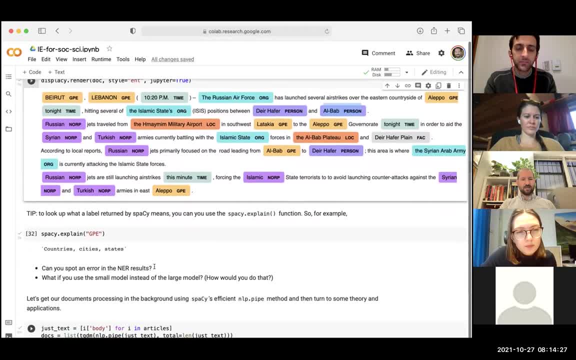 Right, Great. So I think an exercise I'll leave for later is if you you can go back and redo this with the small model as opposed to the large model and see how that affects things. If you want to get fancy, you can also start timing it to see sort of what the trade-off. 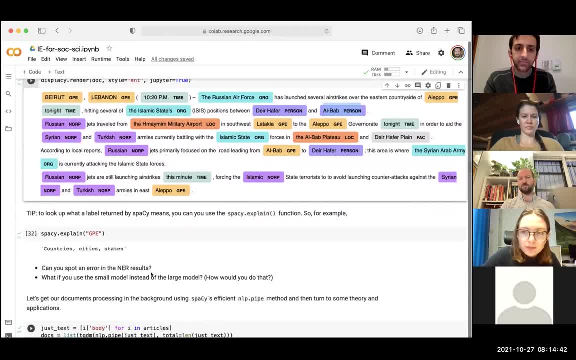 between time and accuracy is but this. it's interesting to to play around with a few different models, especially in your work, where you know maybe you have a million documents and accuracy is not so important, or maybe you have 7,000 and accuracy is very. 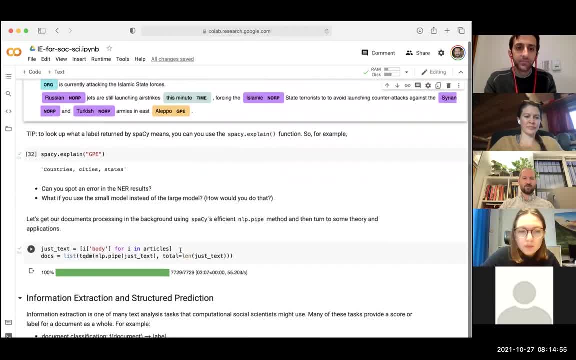 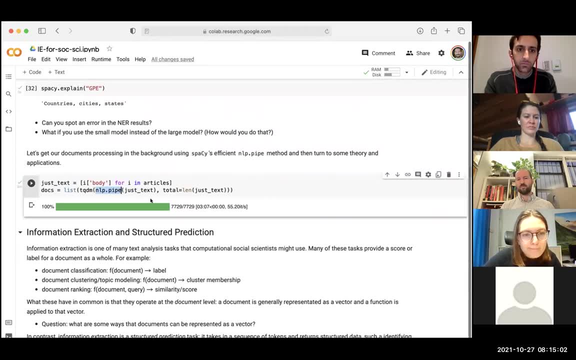 important. Okay, So we're going to get some articles processing in the background so that we can use them later, And Spacey provides this efficient NLP dot pipe method. So this is essentially batches articles together, batches text together, So it can it can do some sort of optimized matrix operations. 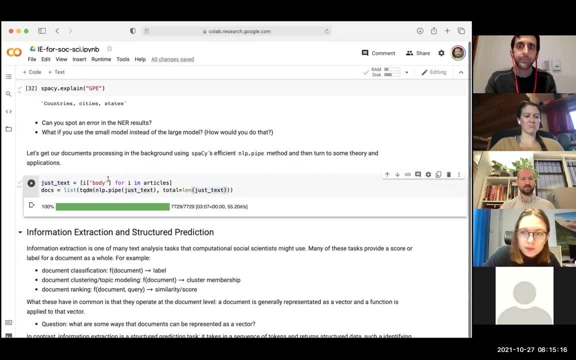 And so this will be noticeably faster than just iterating through the documents by hand, Right? So we're going to pull out just the text- That's all we're going to use for this, this demo, And then Put it through NLP dot pipe and then use one of my favorite things- TQDM- to get a nice 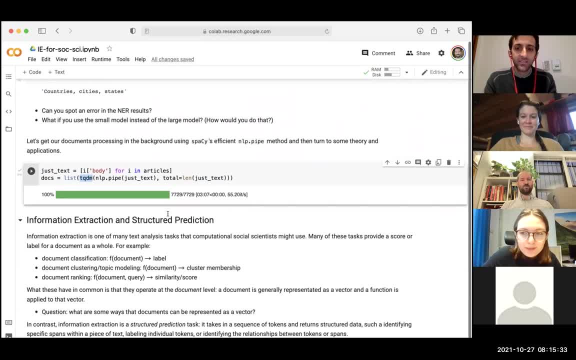 progress bar on it. Okay. So that's sort of what it looks like in practice. we have a document, We get some NLP information- some of it's right, some of it's wrong- But we're in large part adding information at the token levels that we can pull things. 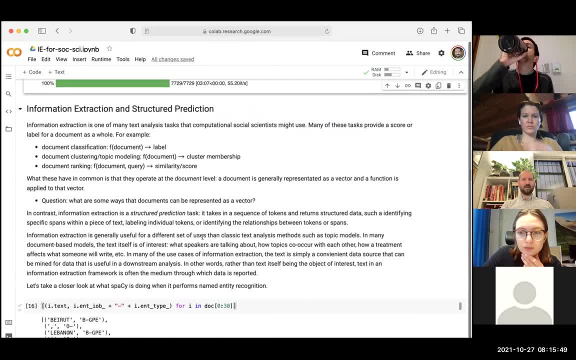 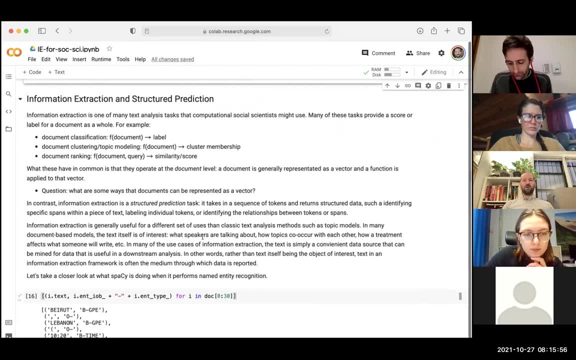 out of a document, All right. So let's let's step back and talk a little bit more Generally About information extraction and structured prediction. So I think people- people in the tutorial- will be quite familiar with a lot of text analysis techniques. 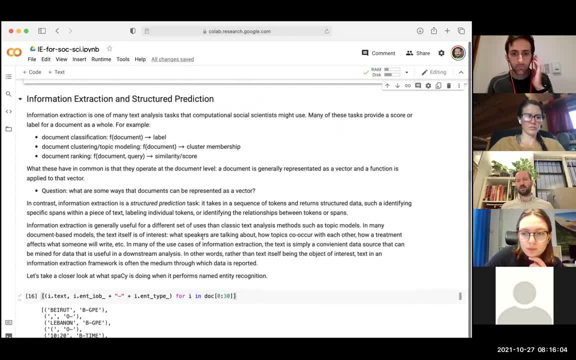 And I think especially in social science, a lot of these operate at the document level right. So document classification is a is a totally standard task that I'm sure many of us have done, And essentially we take in a full document and we want a model to, to give us a label. 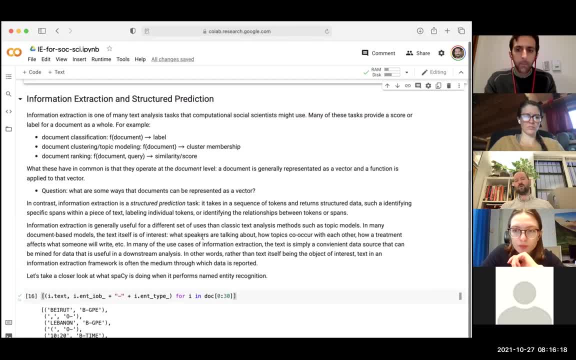 for that document or topic modeling or clustering. We put in a bunch of documents and we get some sort of latent clustering And then we have some sort of a cluster membership for each document out of that model or less common in computational social science, but I think still so relevant sometimes is document. 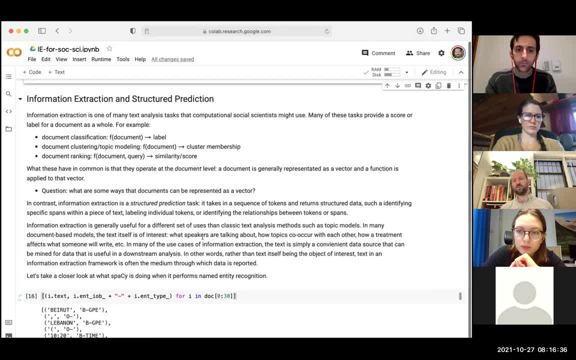 ranking. So we'll- we'll put in a document and a query and get some sort of document level score that tells us how similar that document is to that query. And what all these have in common is that they operate at the document level. 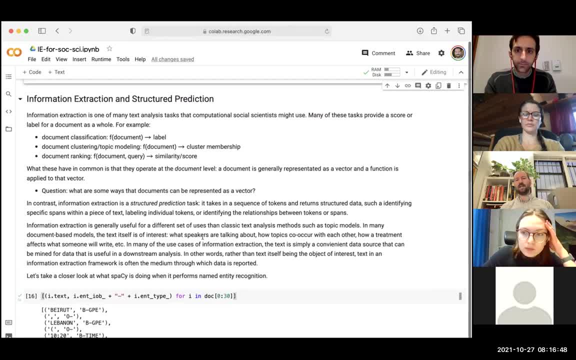 And so a document comes in, we process it and an answer for label comes out for that document. So at this point I wanted to stop and ask, sort of to check on how people are doing, what are some of the common ways that we represent documents as vectors? 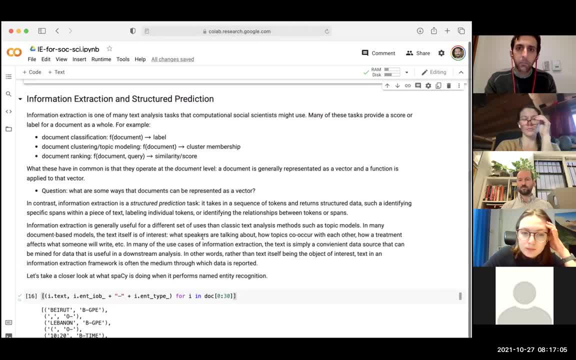 sort of in this document level processing framework. Can you rephrase your question? maybe, Yeah, so when we're doing any sort of text analysis, any sort of computational text analysis, we have text and then we want something out at the end. 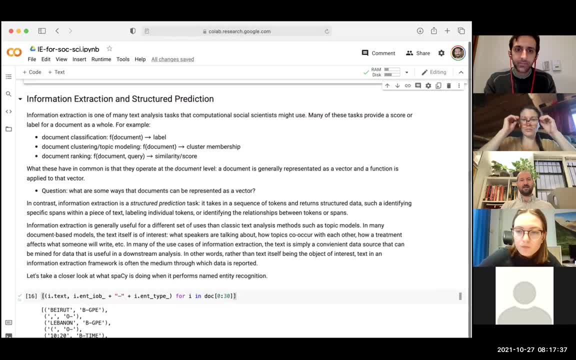 like a label for the document, And in between we have to decide how do we go from a news story to some sort of numerical representation that the computer can operate on. So there are a bunch of decisions that I think we often have to make. 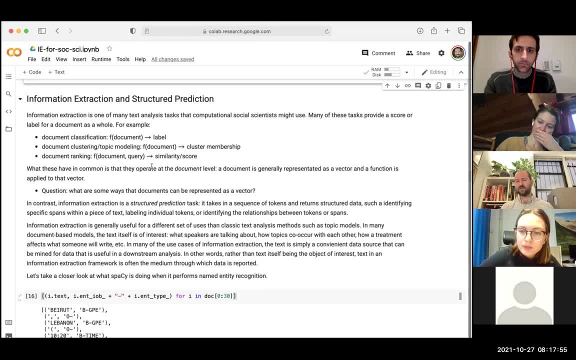 about how we want to represent a document as a vector, And by vector I just mean sort of a numerical representation of a piece of text. Well, in the case of the topic modeling that you already mentioned, we can have like the distribution of the probabilities. 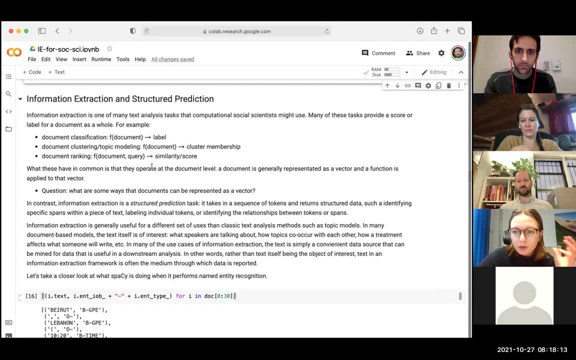 for every topic that we can have for the core project we are working with. Yeah, exactly, So that's what we'll get out at the end of a topic model. is it's going to give us sort of plot, the document on a topic simplex? 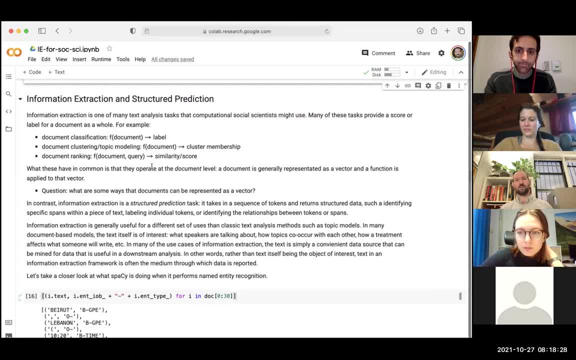 or give us the proportion of topics in the document. But what about before? How do we put the document into the topic model? In the chat? we have Word2Vec too. Yeah, okay, So Word2Vec is one that Anastasia. 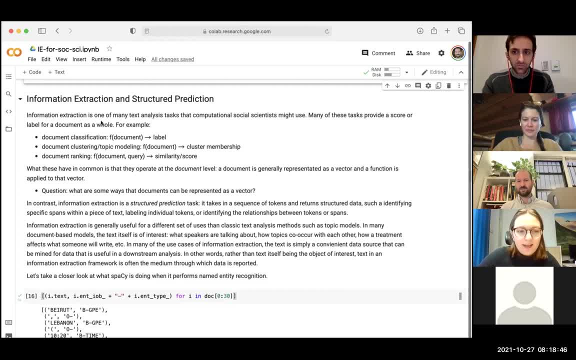 I think you're about to say something too Like. if I understand where you are heading, it's just like the word frequencies that we have in the doc and then the document. Yeah, exactly So we have word frequencies, So we count the words, we ignore their order. 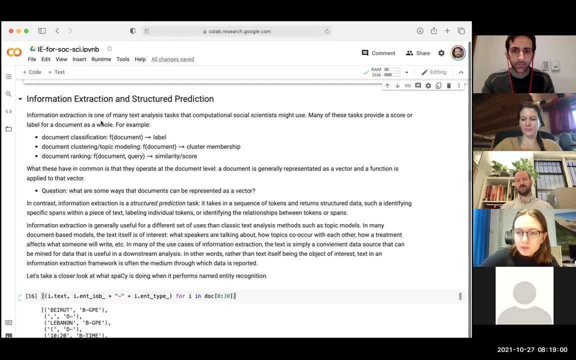 we make the bag of words assumption and we're trying to say this document is represented as counts of different tokens or different words, and then we're going to apply a topic model. So yeah, and so Word2Vec is also from the chat. 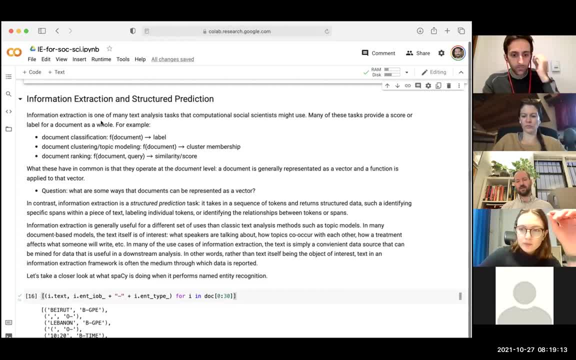 Word2Vec is another way of doing this. We can take a document in, we can look up the pre-trained embedding for each word and we can average them or take the element-wise max or some combination of those and represent them. 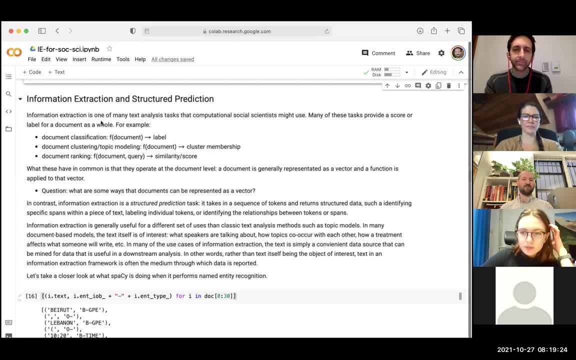 And represent a document as a single vector and then apply whatever function we want to give us: a label, a cluster, membership or so on. So, in contrast, information extraction is not operating at the document level most of the time. It's usually operating at something like the token level. 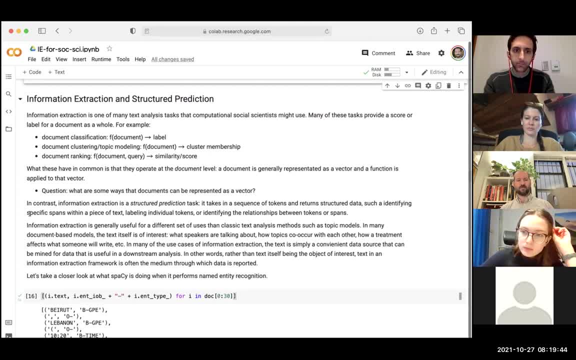 or I think now less commonly, at the character level. So when it's taken in a document we're almost always going to preserve the order of the token And what comes out at the end is not necessarily a document-level label or document-level cluster membership. 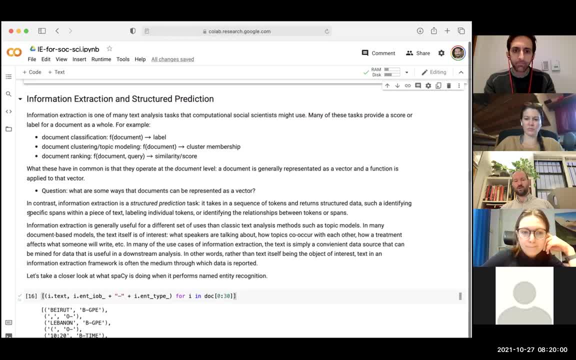 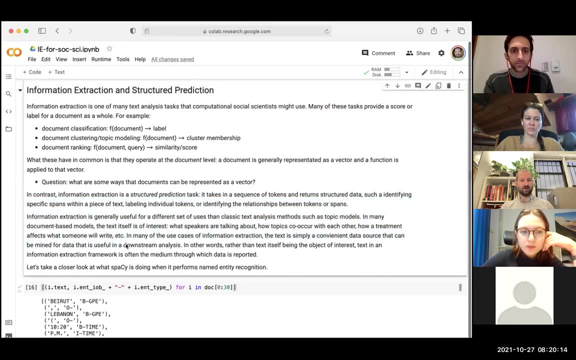 It's going to be a phrase or a word or some sort of sequence of outputs that we're getting from the document. So, yeah, I think I'm going to come back to this note at the end. I just said it in the morning. 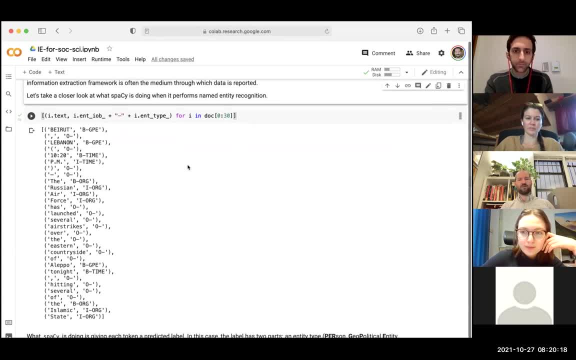 But yeah, so let's look at what that looks like when we do named entity recognition. So we're going to go and just look at the first 30 tokens of the same document we've been looking at And for each token in that sequence of the first 30 tokens. 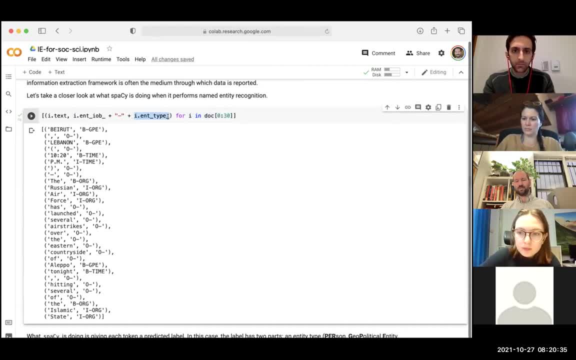 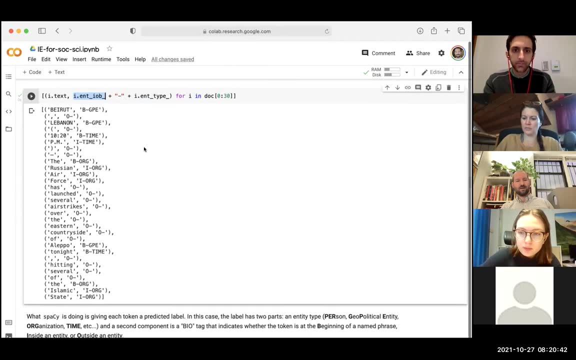 we're going to look at two things. First is the entity type, So these are the same labels we saw earlier in the display, And then we're going to look at the second thing, which is the end: IOB. So I think the entity type is pretty self-explanatory. 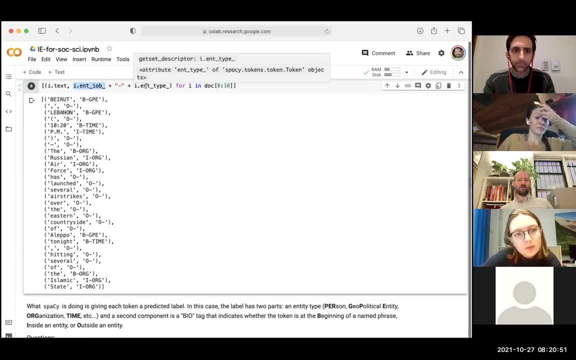 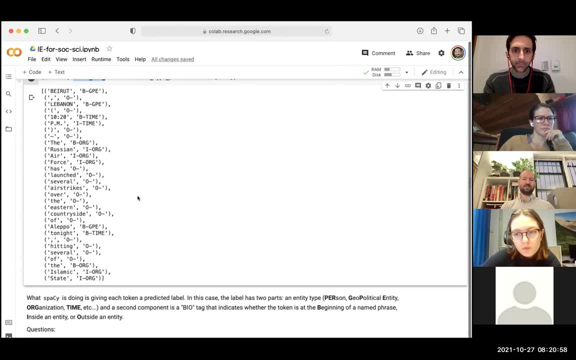 It's things like: is this a person or an organization or geopolitical entity? And the IOB label is a little bit, maybe less intuitive. So in this case, what it's doing is this IOB or BIO tag is indicating whether the token is. 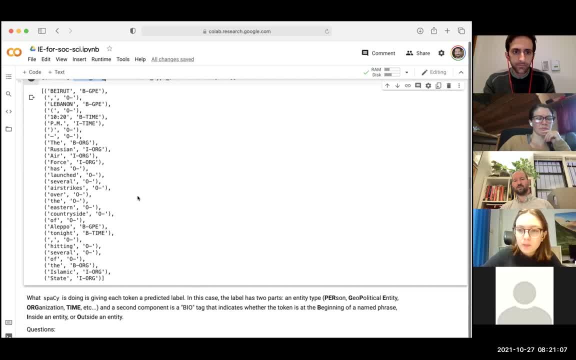 at the beginning of a named phrase, inside a named phrase or outside a named phrase. So here, Beirut is a geopolitical entity, That's correct. It's a city, And in this case it's the beginning. Then the comma is nothing. 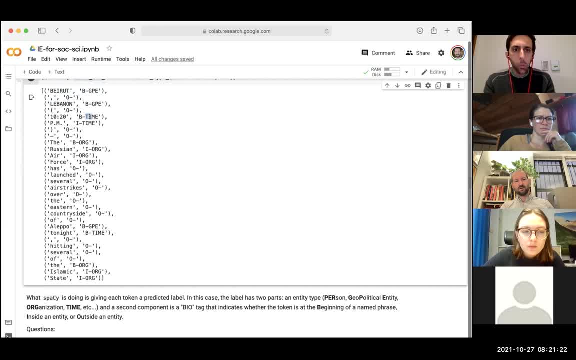 Lebanon is the beginning of it- Geopolitical entity, And then here we have 1020 PM. So both of these are time tokens. In this case, the first one gets the B label at the beginning, The second one gets the I because it comes. 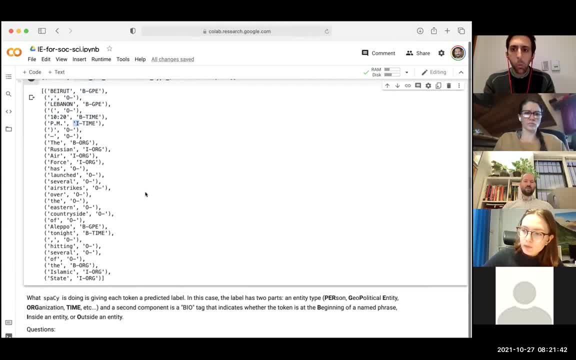 after the beginning, So at a high level. I think what this is meant to demonstrate is we're still in some sense doing classification. We are doing classification here, It's just at a much more granular level than when we're doing document classification. 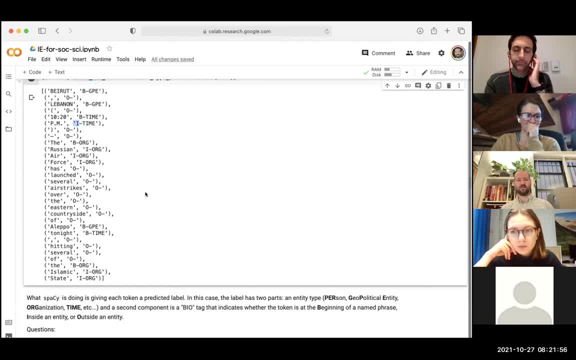 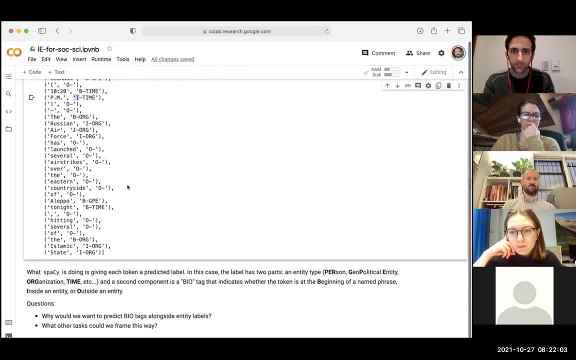 So we're trying to assign a label to each token so that we can do something else with those tokens. So just sort of starting to think about representing documents and word order and structures. Why would we want this BIO tag or this IOB tag? 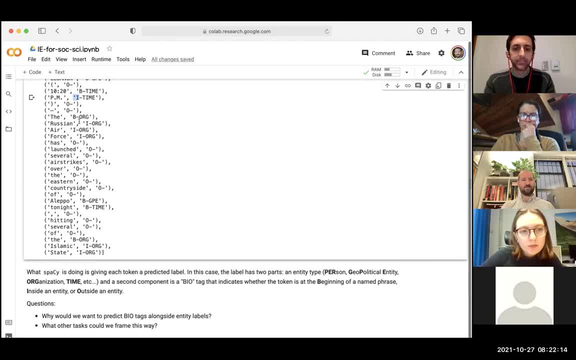 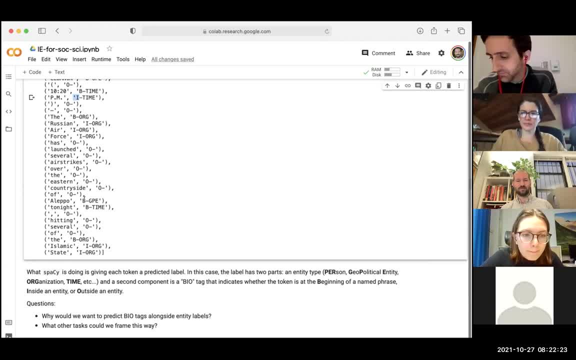 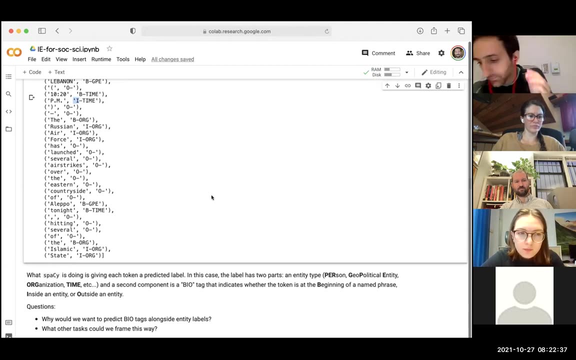 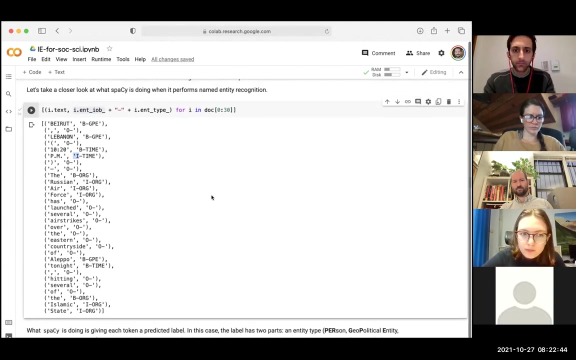 Why? why do this BIO thing at all In the chat? we have different orderings, can have different meanings, Yes, So say more about that, Nina, if you want to. I was just thinking in terms of the way in which, if the root is like paired with something, 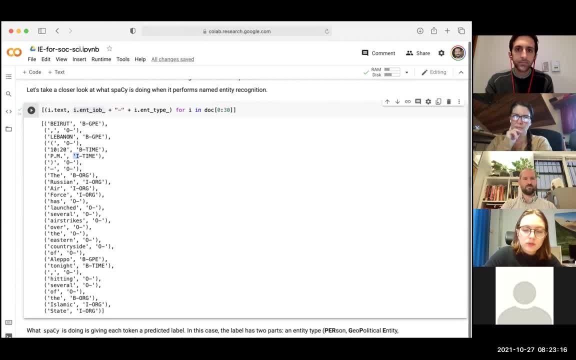 else, or if it's like at the beginning of the token, it might have a different meaning depending on. I mean, that's probably a bad example, but I guess Russian, whether it's at the beginning or in the middle, might be might be important. 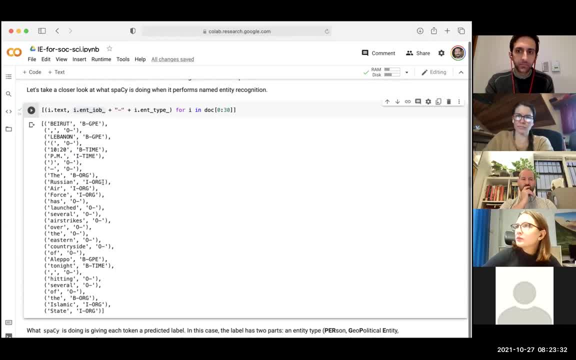 Yeah, Yeah. So I think I think what you're getting at with that is, you know, the the label GPE can mean different things, right? So essentially, we could have a situation where we have We have two different GPEs mentioned right next to each other. 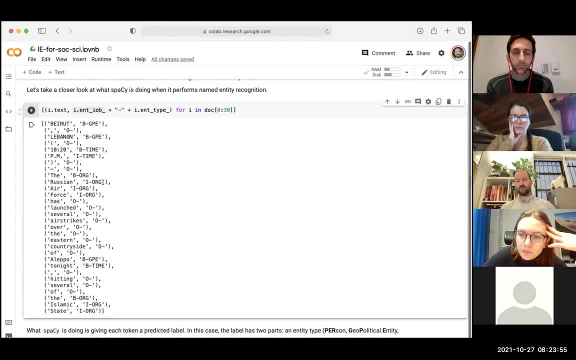 And if, like we could have, you know, a Russian American summit and in that case, you know, if, if we don't have the beginning and inner, we don't know if Russian American is is one nationality or if they're two separate nationalities mentioned alongside each other or like the 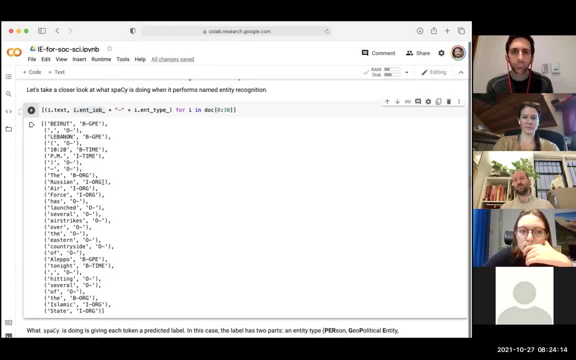 New York- Boston train is. is new a city, York a city in Boston city, or is New York a city, a city in Boston? Right, So this, this BIO helps us to keep track of of some accounting, I think, sort of at a. 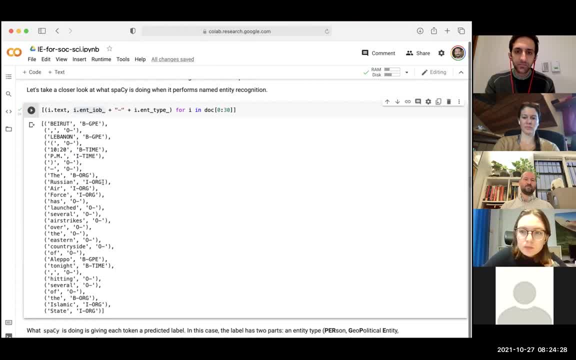 thing in a different way. I think there's- I think there's- some pretty good research that also predicting these labels alongside the actual entity labels helps increase the accuracy. So the model begins to learn things like this. This is a good signal that a that entity is is starting. 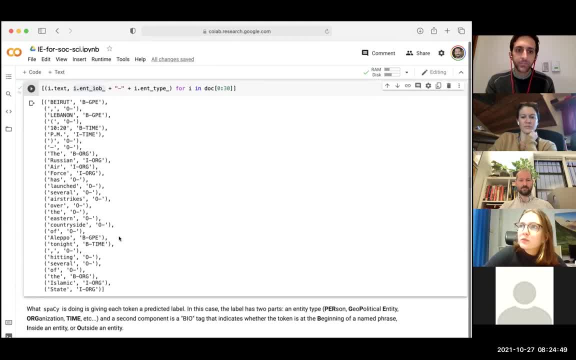 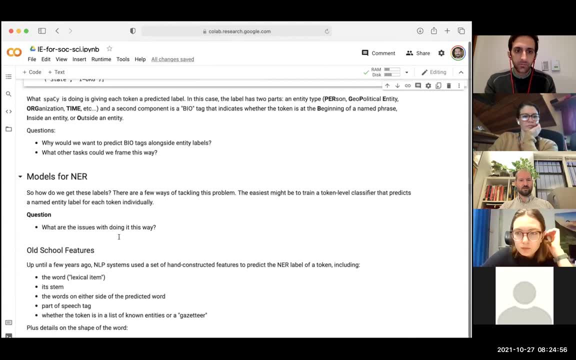 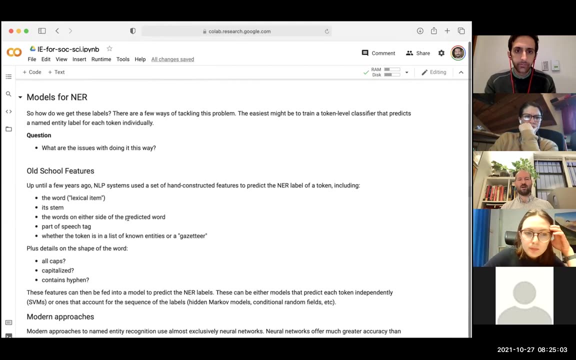 And then this is a good one. It's continuing, Right, Yeah, Okay. So that model discussion, I think, leads into sort of a another discussion about what are like what? what are the models for NER? How do we get these labels? 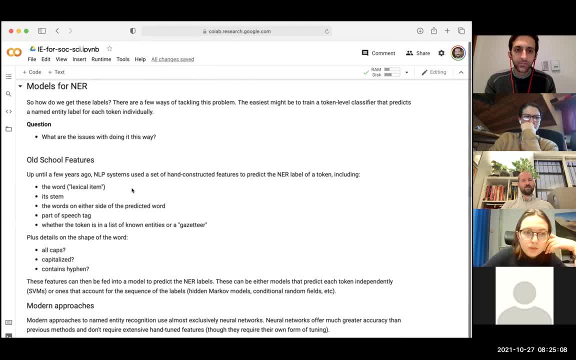 And I'm I think I'm gonna go pretty quickly through this because I think this is something that you can. you can look through on your on your own later. But one option is: we can, we can, you know, just kind of. 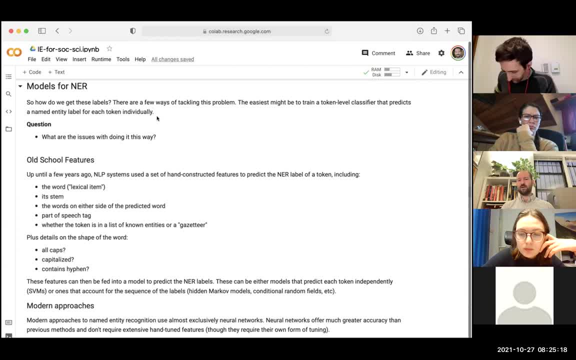 Yeah, Yeah, Just train a token level classifier that that tries to predict those labels, right, So we can. we can ignore the words around it and just say, you know, predict this label for for each token. And I think, as as we were starting to talk about it before, one of the issues with this: 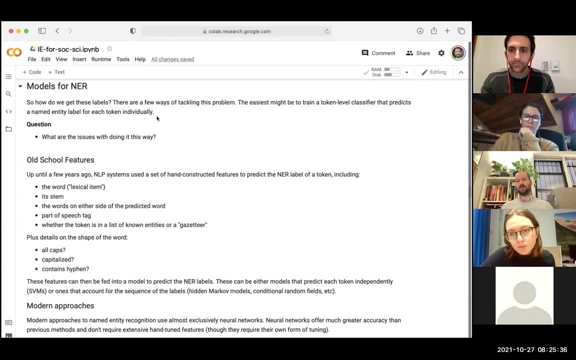 is that there's a lot of dependence between the labels that we predict, right So so it's impossible to have the an I label at the beginning of a word, because that's that's sort of against the rules, Right. 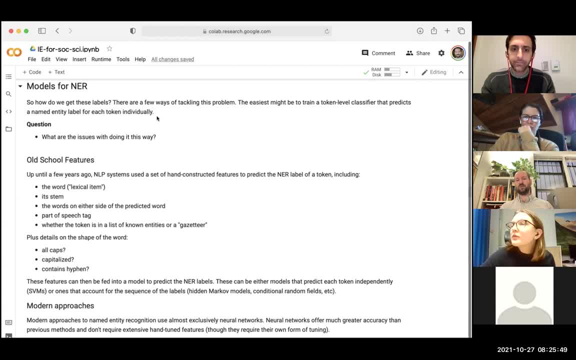 So, but once we've seen a, B, so beginning of an entity, the next token is more likely to be an entity of that same type than just a randomly selected token from elsewhere in the document. Right, So there's there's a lot of dependence between tokens and a lot of the models that people 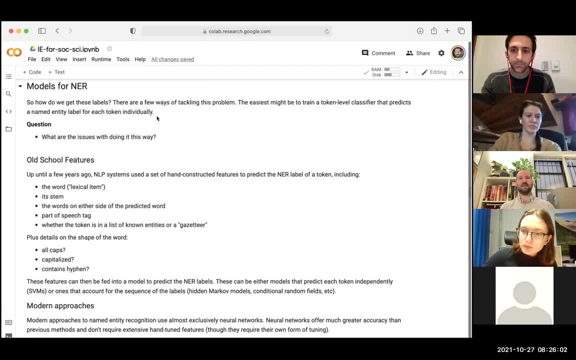 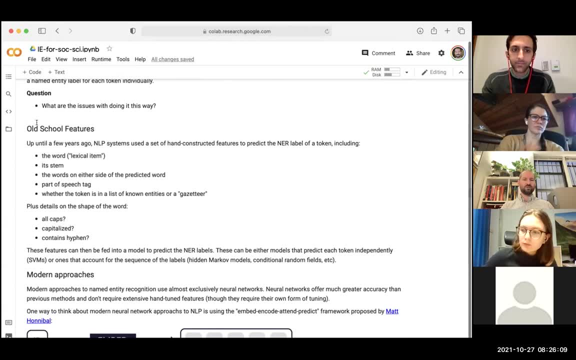 use are ways of of making sure that that that dependence in predictions is preserved through the to the final prediction, Right? So so old school- and Ian was laughing out, that's when we talked about it last week. So old school meaning like six years ago. 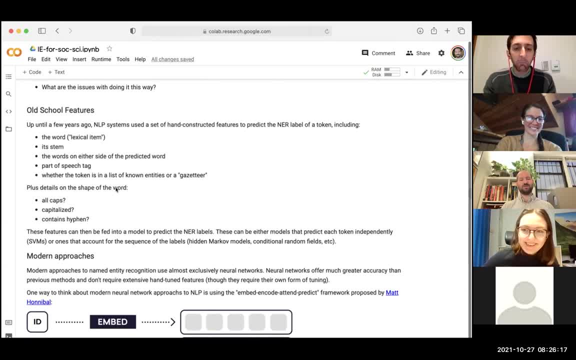 This is the way that That people used to do the sort of token level tagging task right. So people would. would create all these different features for a word, like the word itself and the words on either side, And is it capitalized or does it have numeric, or how long is the word. 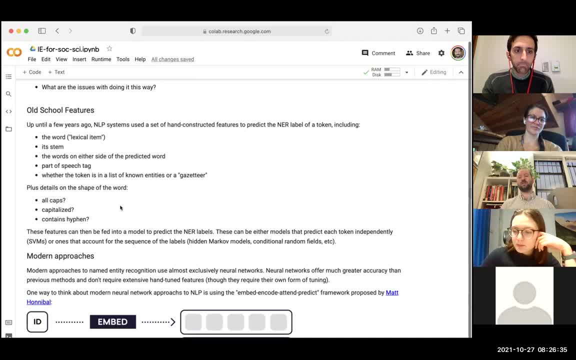 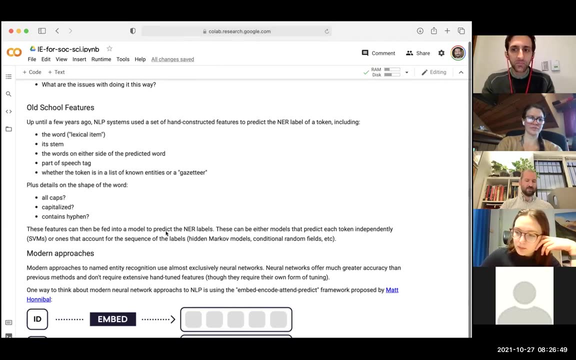 Does it contain a hyphen and then put that into something like a support vector machine to predict the token label for each, each token. the sort of the more modern approach almost always uses Right, Right, And so I think there there are a couple of reasons for this. 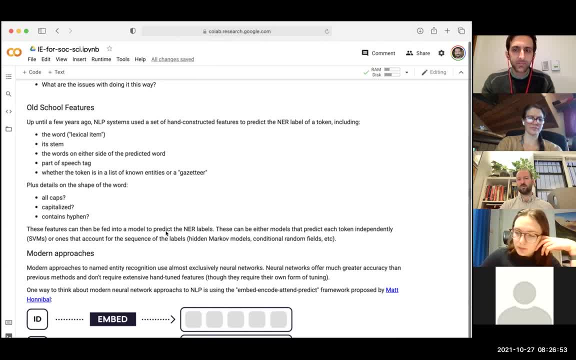 One is is pragmatic. They they just tend to perform better than the, than the older approaches for for things like named entity recognition, And also there's less sort of. there's less need to hand tune all these features, although of course neural nets require their own, their own forms of tuning. 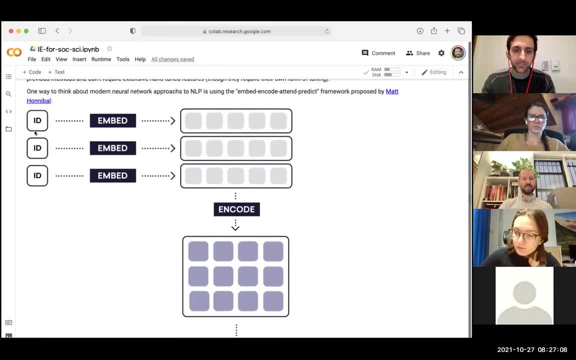 So this is a figure that the, the person who is the lead developer of space, he wrote, but I think sort of a nice overview of what a neural net is doing And I'm not going to get into the details of this. There are lots of good blog posts. 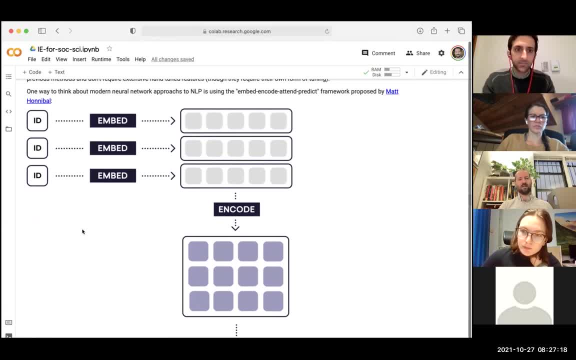 That will explain things like this, but sort of as a high level. I think this is a conceptually useful way of of thinking about something sort of this: the neural net approach, right. So we have a sequence of tokens that come in, and the first step is we embed these. 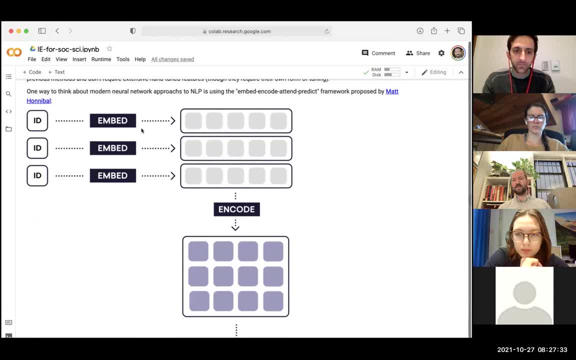 So in a lot of cases this is using something like like glove or word to net, word to vec. So we're looking up a pre-trained embedding for it. So a word ID comes in and then we we now represent it as a dense vector. 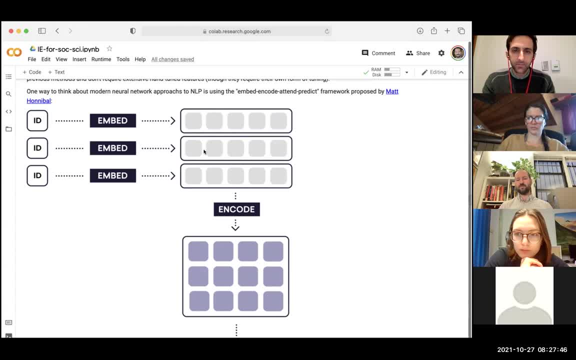 But each of these is independent, right, So we were not accounting for the context of a word or the features on either side, And so a common second step is to do something that he calls encoding. we use the term encoding to refer to. 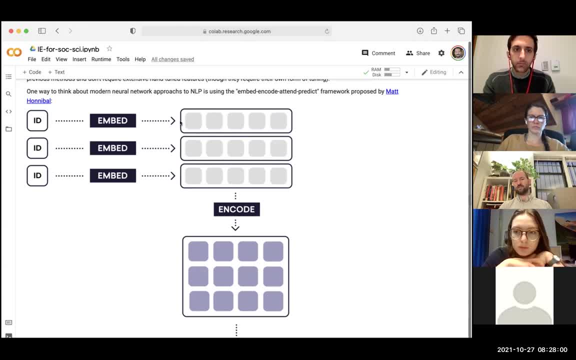 So this is a way of taking these independent tokens that we've represented as as a vector and changing the representations that they account for context And there there are many different ways of doing this. Things like recurrent neural nets, or LSTMs, if you've heard of those, are one way of doing. 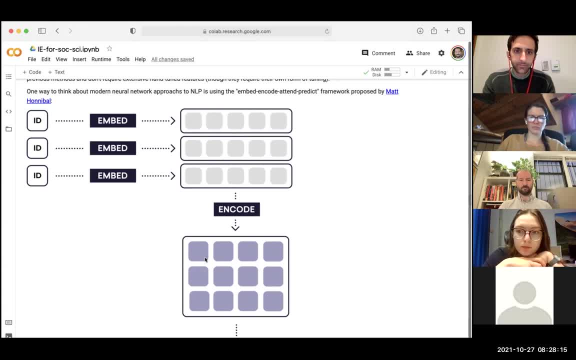 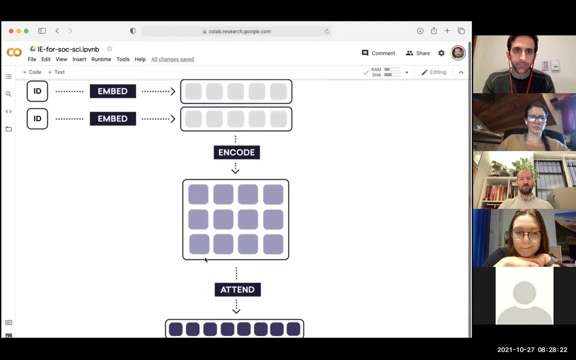 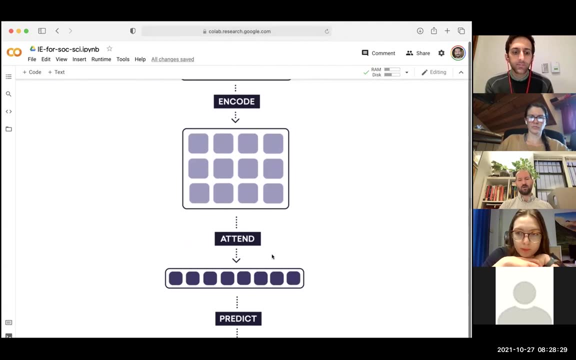 it And transformer models are are a different way of doing it. All right, So we want to change our representation of of a word to account for the context of that word: The. the next step in this, in this framework, is is to attend, and I'm not really going. 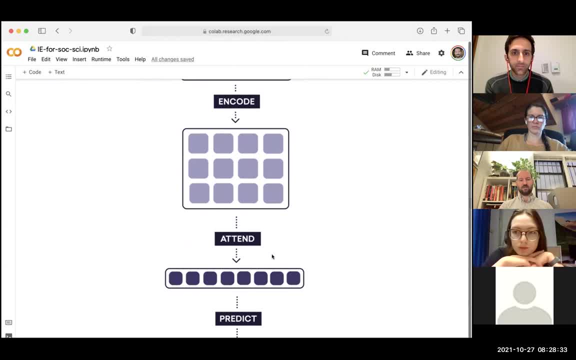 to go into depth on what this is, but this is one of the features that that underlies: sort of modern transformer approaches, which are sort of a class of models that are performing very well on a lot of NLP tasks And sort of the the high level. 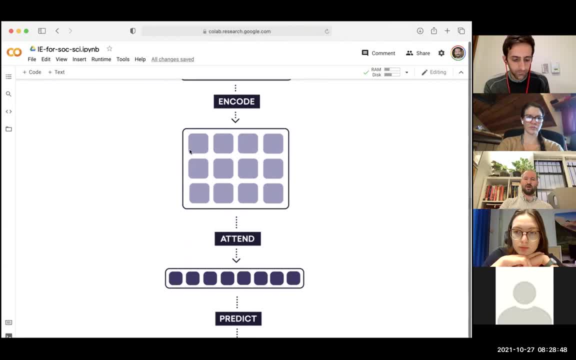 One of the advantages of this sort of set of outcomes for today. The other thing that we're going to do is we're going to go into a little bit more detail here in just a few minutes, but we're going to go over this one thing: that that is a. 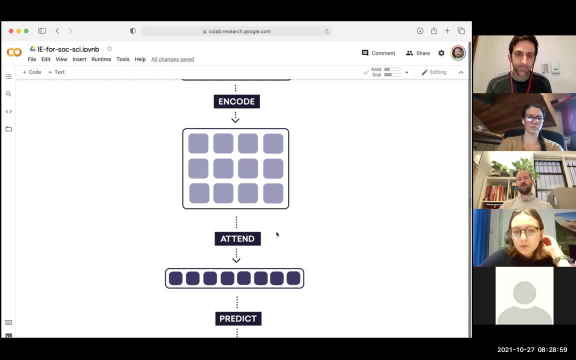 bit of a follow up to what we set up in the previous slide. for a little bit, here is we. we often need to make a prediction, Sort of for a specific token in this sort of encoded collection of information and attention is one way of learning, not only sort of how do we represent words in contexts? 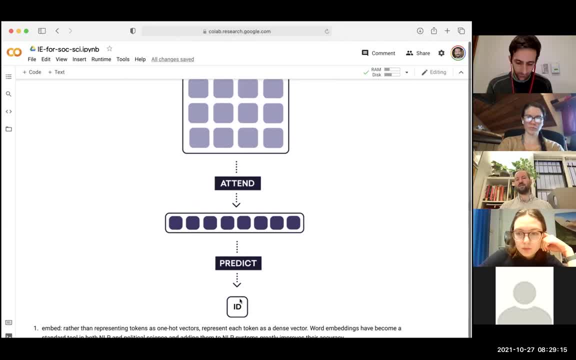 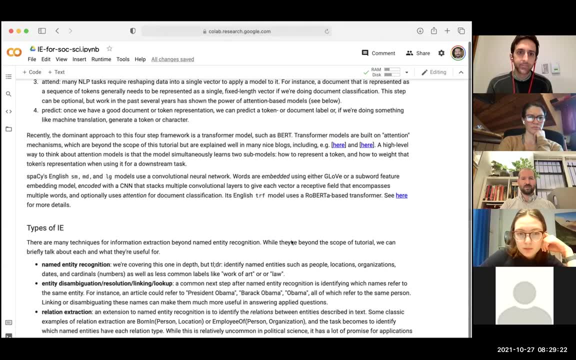 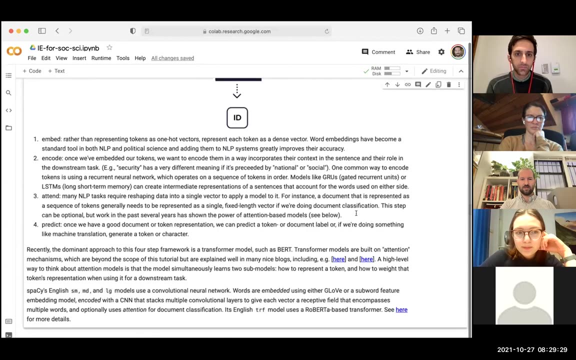 but also, when we're making a prediction, How do we wait? learned contextual weight that we apply to our, our document representation. so that that's a high level explanation. uh, other people have explained it better, i think, with much better pictures. um, so i'd highly recommend uh reading these- sorry, uh, these blog posts here, which they do a very nice. 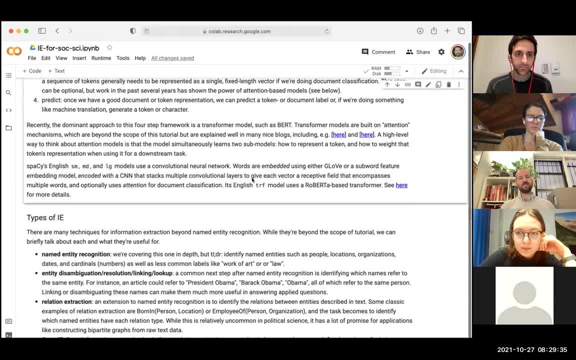 job of explaining how how these work. so spaCy uses a convolutional neural network as the way of getting token level context. so, um, it's, it's going to look um sort of not at all the words in sequence, uh, but sort of looking at words on either side and then sort of gradually expanding out as 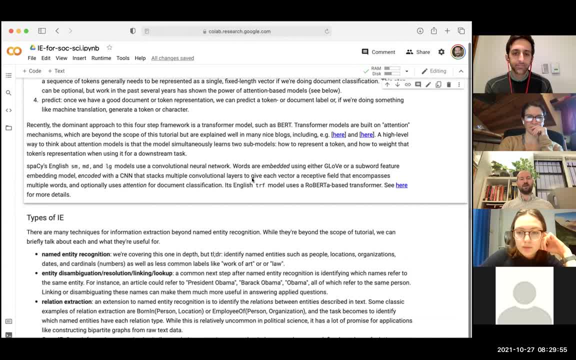 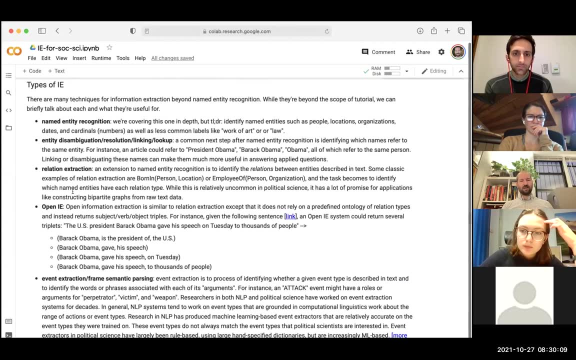 the layers go deeper, so it's it's still encoding the context into the way that represents, um uh, each token. so there are more details here that i think you can look at at your leisure, okay. so that that's that's sort of generally at a high level, how the models for these token level models. 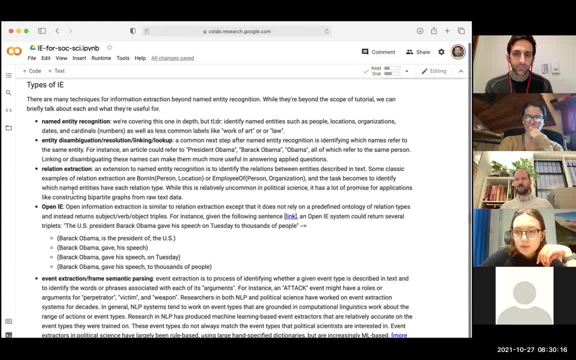 work. um, i'm i think, in the interest of of time, i'm going to go pretty light on sort of the whole world of information extraction because i want to get to the demos and the hand on hands-on part. but i think the thing to take away here is what we're doing. 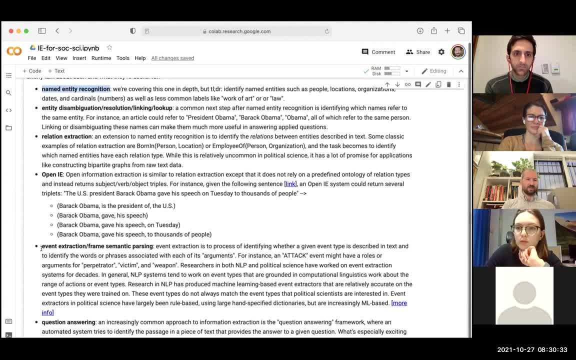 named. entity recognition and the sort of light event extraction are just two different things in a pretty big universe of information, and one, isとапom, is a really popular sort of innovation in the field when we're looking at one of the most dangerous things that we can play with these things. um are patterns, and one of the key things in the 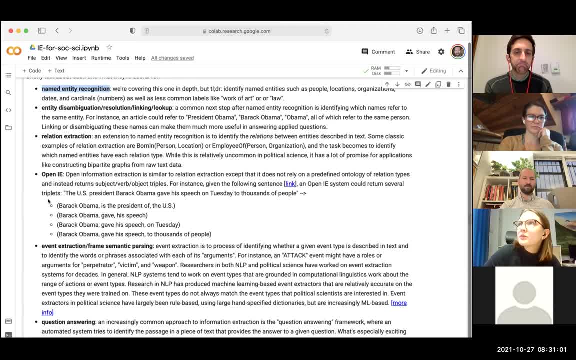 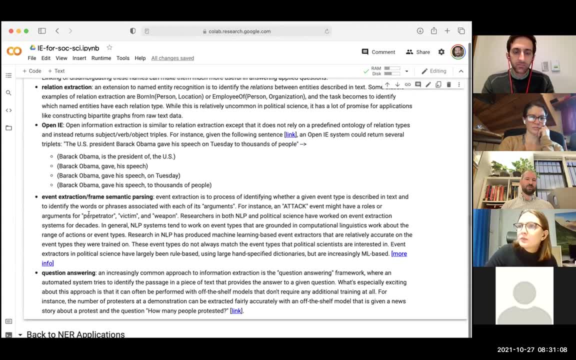 play on photoshop is figuring out what's on. what are different pseudo metaphors of these drug mechanisms that you can do? there's going to be a set of ways of sort of clicking through them. uh, these aren't general, which is what my research is on, which is, when we have a document, how do we identify? 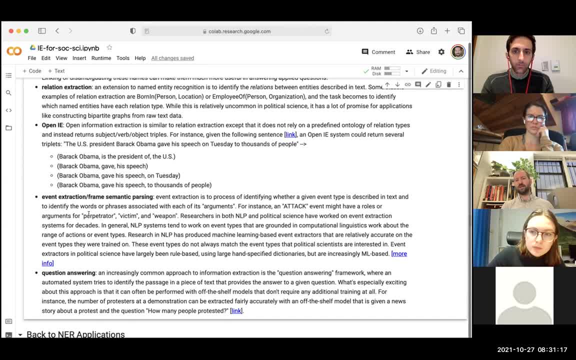 complete events and all the attributes of events in there. So who's doing an action, who are they doing it to, how are they doing it where, and so on. So these are all different ways of doing information extraction in social science and we're just going to focus on two. 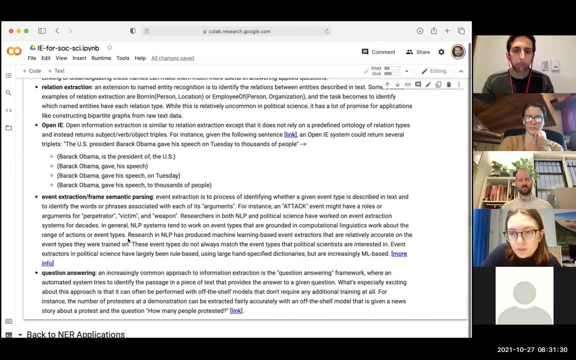 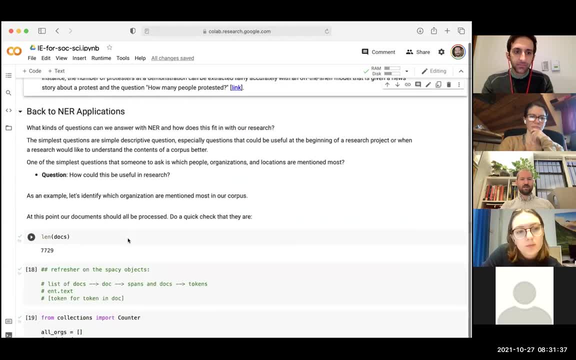 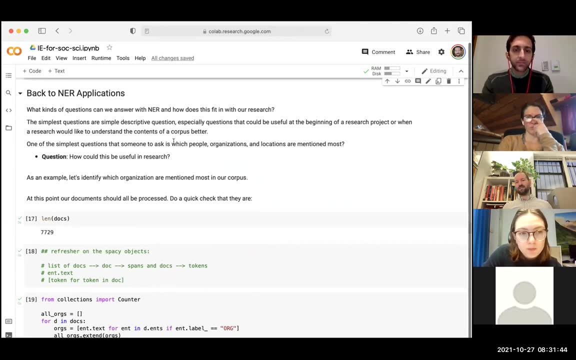 of them. now named entity recognition and then using dependency parses, which I'll talk about more later, as a way of extracting information. Okay, back to the NER applications. So yeah, so named entity recognition essentially gives us the named entities and the documents of the. 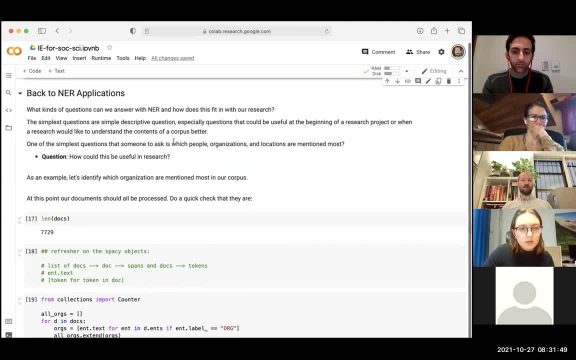 people, the organizations, the locations and so on, And the simplest questions that we can answer with this are essentially descriptive questions, right? So who's mentioned in this corpus? how often are they mentioned, and so on, And I think you can. 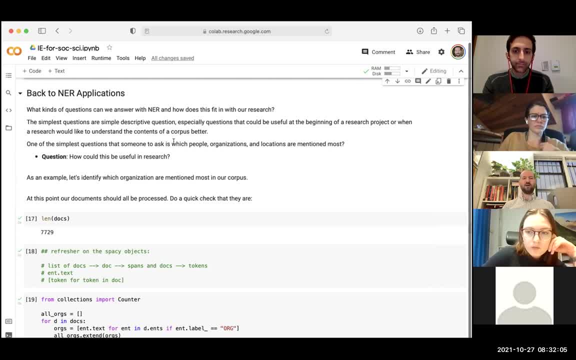 think of this as a way of looking at it from a different perspective, right? So who's mentioned in this corpus, how often are they mentioned, and so on? I think you can all think about how that could be useful in your own research, but I think oftentimes it's useful. 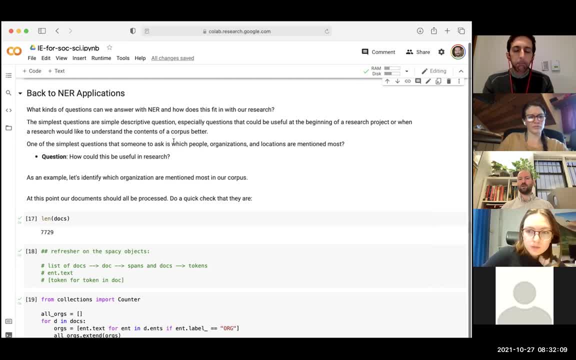 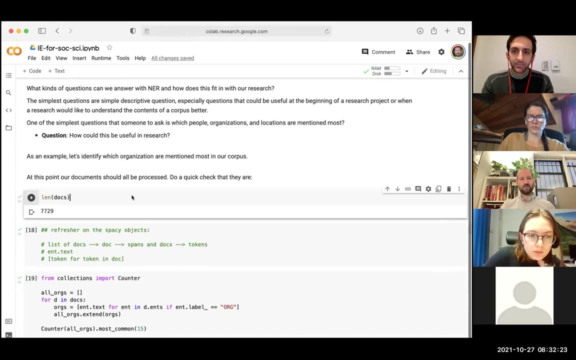 in earlier phases, or an exploratory step or as a way of you know, exploring what's in your corpus before you do something a little bit more directed. that will give you the data you need to answer your questions. Okay, so if you're following along on your notebook, you should be able to run this. 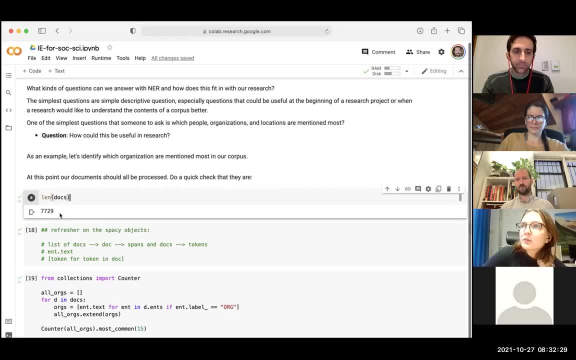 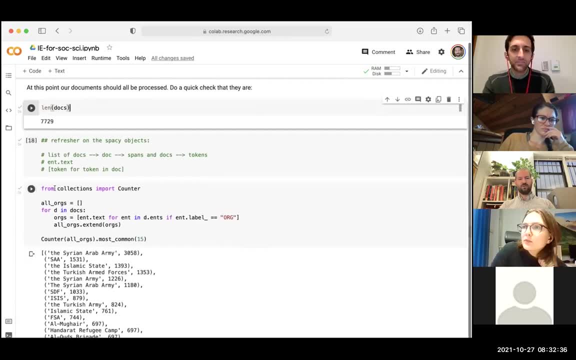 and see that the documents are processed and that you should have the same number that I do. Okay, So the first thing we're going to do is just see, in this large corpus of, or smallest corpus of text, who, which organizations are mentioned the most. 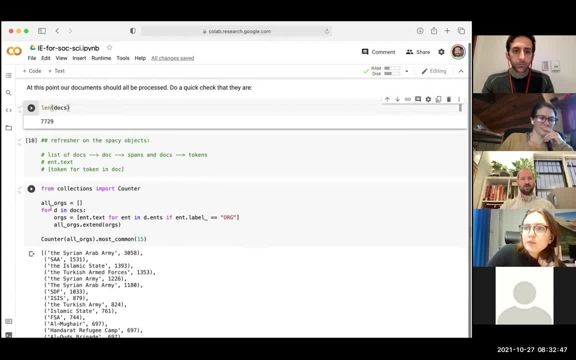 Okay, And the way we can do that is we can iterate through each of the documents. So for each document D we can go through the entities in that document. So in the document there's this ends attribute, We can iterate through each of them And if it's an organization, we can append its text to this. 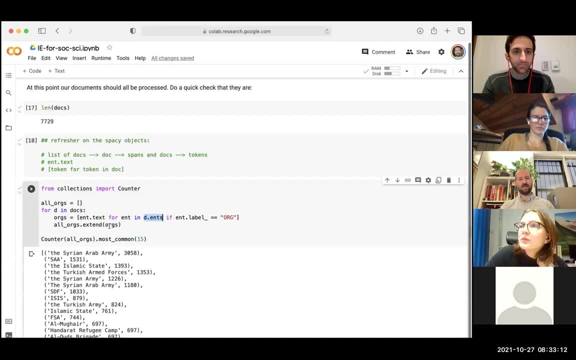 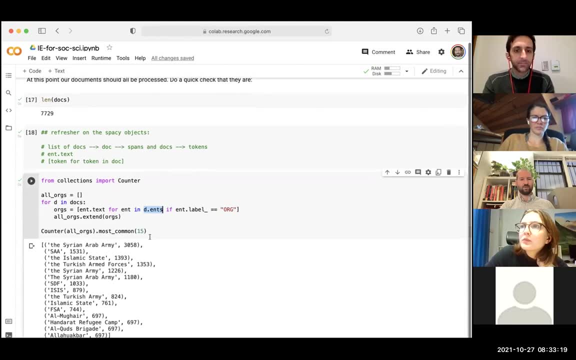 Sorry, Yeah, Create a list and then and then append that or extend that list to a long list and then just use counter as a way of seeing sort of which ones are mentioned most often. So if we look at the most common 15,. 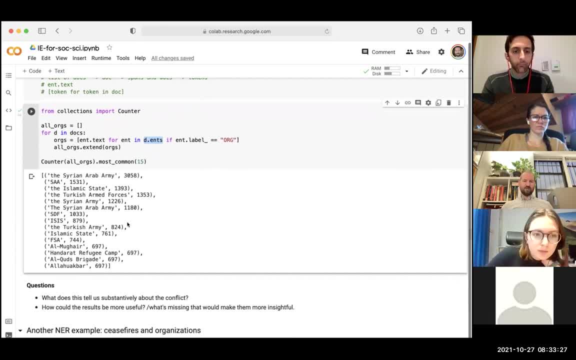 this is, this is what we see, All right, So. so what does this tell us, sort of subs, substantively About the conflict, Like, even if we know nothing about the civil war in Syria, you know, we, we know some things now, And what do we? what do we learn from this exercise? 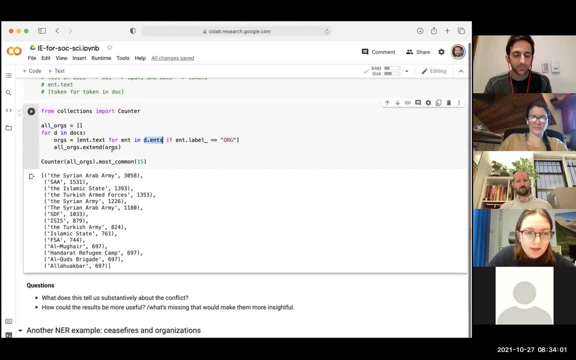 Well, we actually get like: what are the participants and what do we learn from this exercise? And I guess how often they are, how often they show up in the texts, kind of shows how active they are, or at least how this particular news source shows them how active they are. 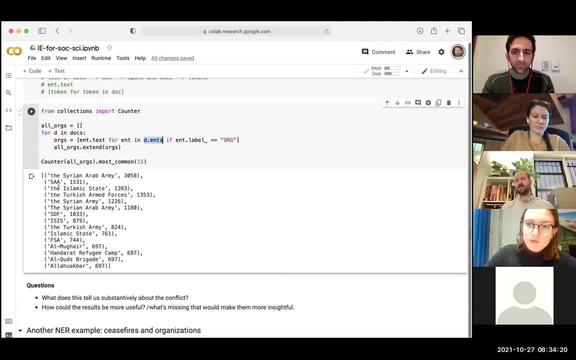 Yeah, exactly So. so, even just looking at this, you know we we'd probably expect that in a civil war, you know the there'll be the armed forces of the country and there'll be some rebel groups. But we also see that the Turkish army is mentioned a lot in this conflict which, if we 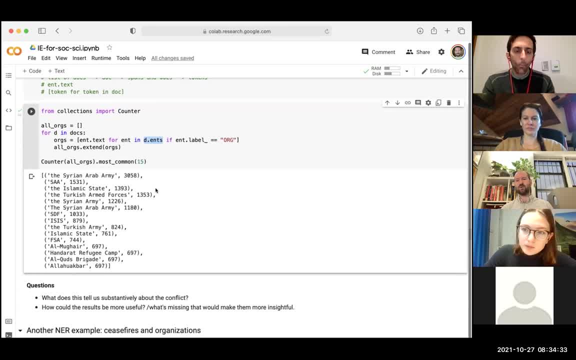 if you know things about the Syrian civil war, this makes a lot of sense. There's the Turkish army is is operating in Syria and during this period there was a lot of near war between the Syrian army and the Turkish army. And then we also. we also see some things that we might need to look up, like if we don't know. 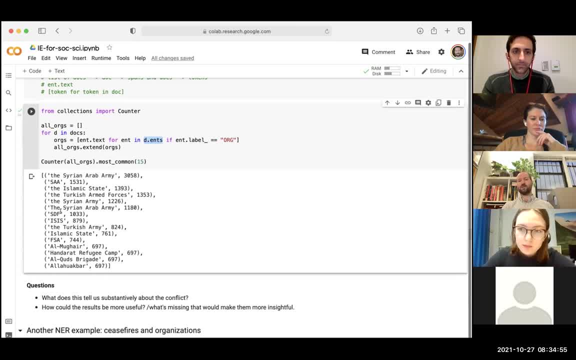 a lot about the conflict. we might need to look up who the SDF is Interesting, And I think this is useful as a way of going and making sure that we understand who all the actors are or what's going on. in our corpus We also see some things that are again errors that the model is making. 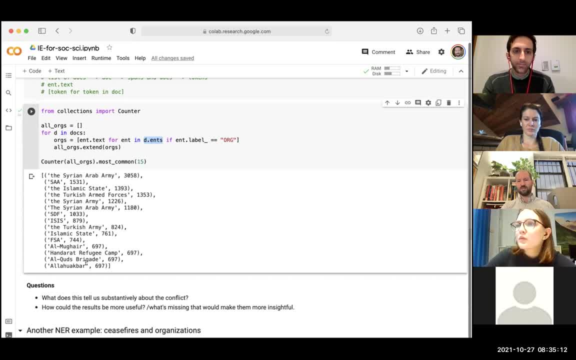 So Allahu Akbar is not the name of an organization, It's, you know. it means God is great, and the sort of propaganda part of this article likes to attribute this to Islamist fighters as a way of making them sound more Islamist or something. 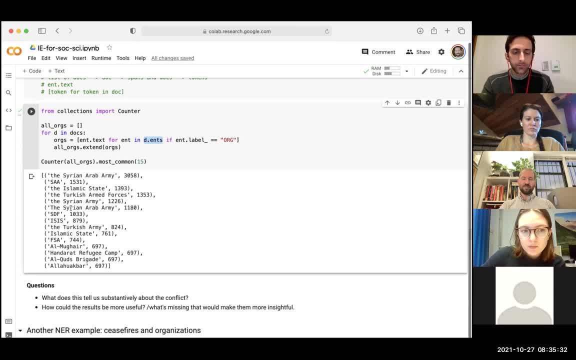 So again here we see some errors that come from taking models that are trained mostly on American and European news texts and applying them to the Syrian conflict, But we also learned some useful things, like who the actors are, who are involved here, One way that this works. 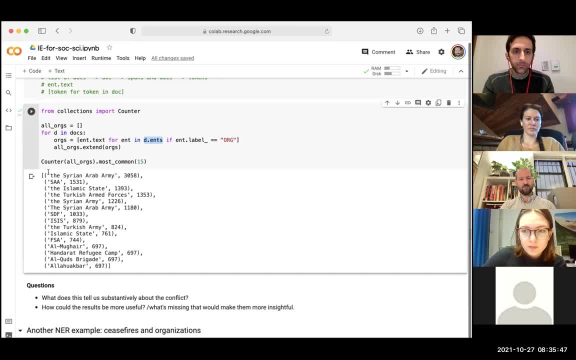 one way that these could be made more useful, you might have noticed, is we see a lot of duplication here. So the Syrian Arab Army, SAA, the Syrian Army, the Syrian Arab Army with a capital T, These are all mentions of the same entity, right? 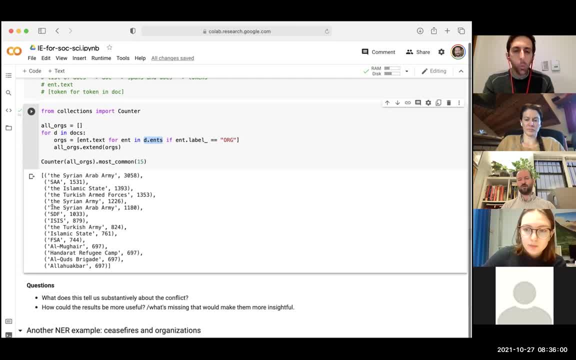 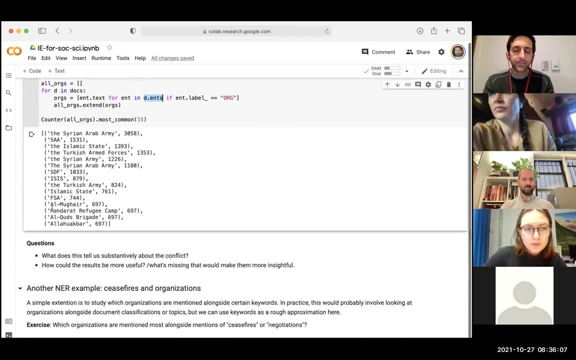 So this is a case where, if we wanted to be more precise, we could have a model that tries to link these all together and sort of say these are all different ways of describing the same entity. Okay, so now I wanted to get to the first interactive part. 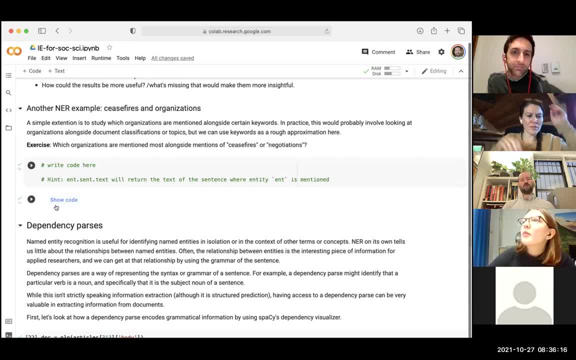 Okay, so now I wanted to get to the first interactive part, Which is we might go one step beyond just who's in the corpus and start to say what organizations are mentioned alongside different concepts or topics. And if we were doing this sort of for real, we might train a document classifier or do a topic model. 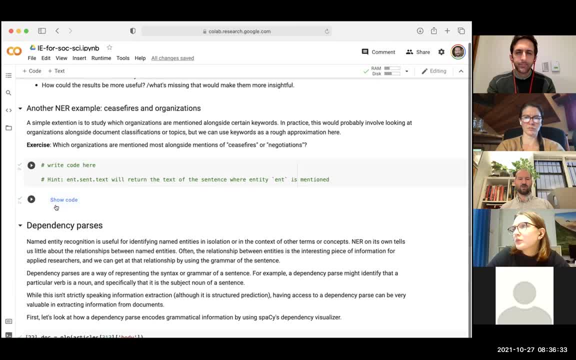 But in this case we can approximate that with just looking at keywords. So I wanted people to have a chance to write some code here and specifically to look at what organizations are mentioned. So I wanted people to have a chance to write some code here and specifically to look at what organizations are mentioned. 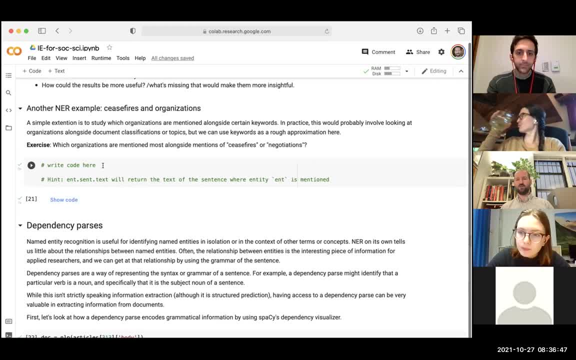 Most alongside ceasefires or negotiations, And with all of these, the answer is right here. If you want to skip ahead and look up one way of doing it, but not the only way of doing it, And with all of these, the answer is right here. 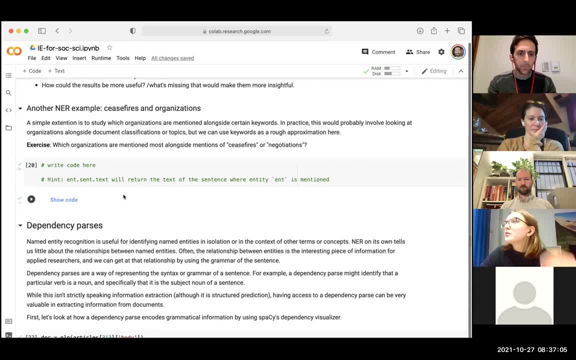 If you want to skip ahead and look up one way of doing it, but not the only way of doing it. And with all of these, the answer is right here. If you want to skip ahead and look up one way of doing it, but not the only way of doing it. 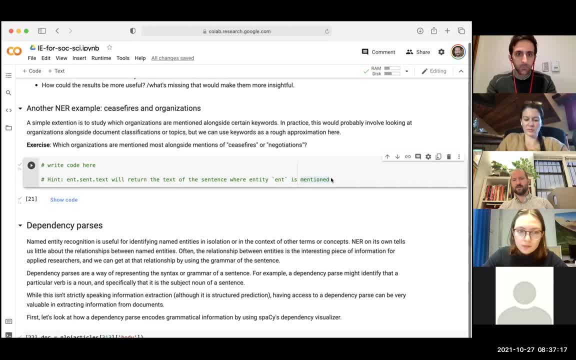 And with all of these, the answer is right here, If you want to skip ahead and look up one way of doing it, but not the only way of doing it. And with all of these, the answer is right here, If you want to skip ahead and look up one way of doing it, but not the only way of doing it. 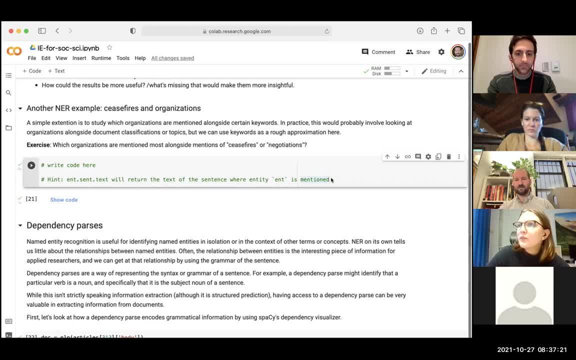 And with all of these, the answer is right here, If you want to skip ahead and look up one way of doing it, but not the only way of doing it. And with all of these, the answer is right here, If you want to skip ahead and look up one way of doing it, but not the only way of doing it. 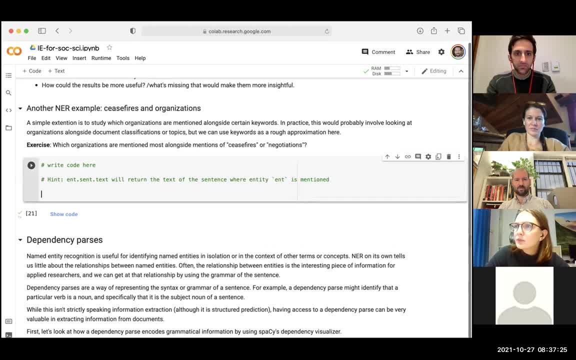 And with all of these, the answer is right here, If you want to skip ahead and look up one way of doing it, but not the only way of doing it. And with all of these, the answer is right here, If you want to skip ahead and look up one way of doing it, but not the only way of doing it. 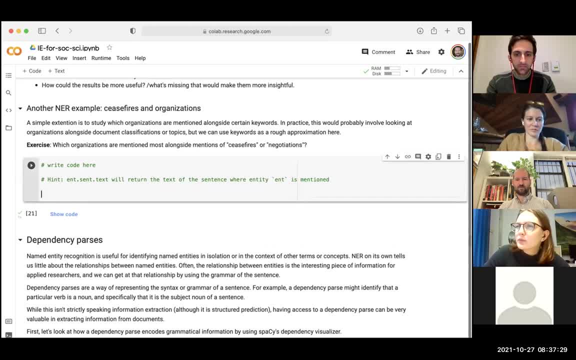 And with all of these, the answer is right here, If you want to skip ahead and look up one way of doing it, but not the only way of doing it. And with all of these, the answer is right here, If you want to skip ahead and look up one way of doing it, but not the only way of doing it. 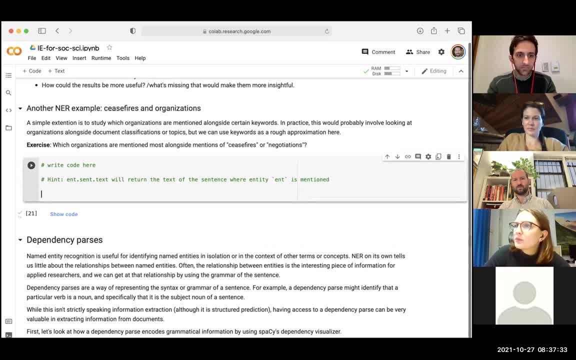 And with all of these, the answer is right here, If you want to skip ahead and look up one way of doing it, but not the only way of doing it. And with all of these, the answer is right here, If you want to skip ahead and look up one way of doing it, but not the only way of doing. 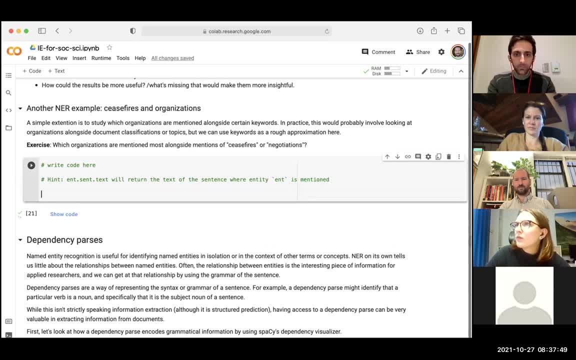 it, but not the only way of doing it. And with all of these, the answer is right here. And with all of these, the answer is right here. Thank you all for your time today. Bye, Thank you. So does anyone want to paste either code or sort of how they're, how they're thinking? 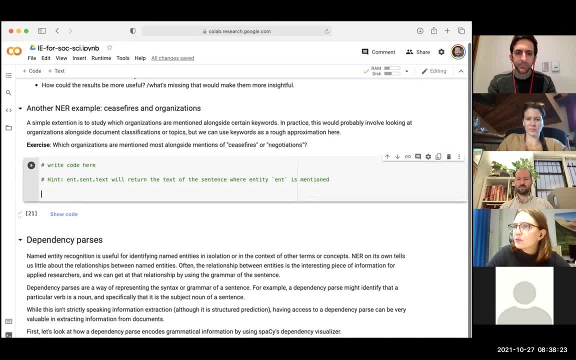 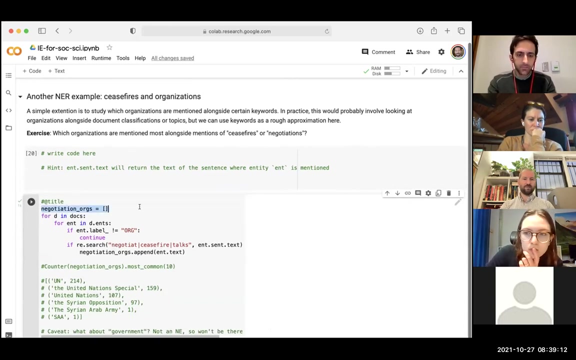 about approaching this. Okay, I'll I'll give it another minute and then show what what I have, and you can go back and work on this at your leisure, Okay so so one way of doing this is similar to above the instantiate a list and say for. 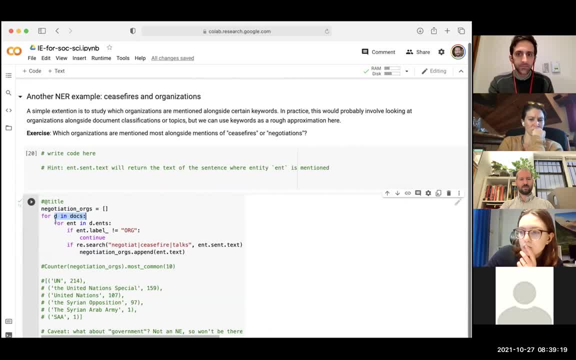 each document And then within each entity in that documents entities. If it's not organization, we don't care, so keep going. And then here we can, we can use regular expressions. there are other ways we could do this. We could check for for lemmas, so sort of about lemmas as being a smarter way of stemming. 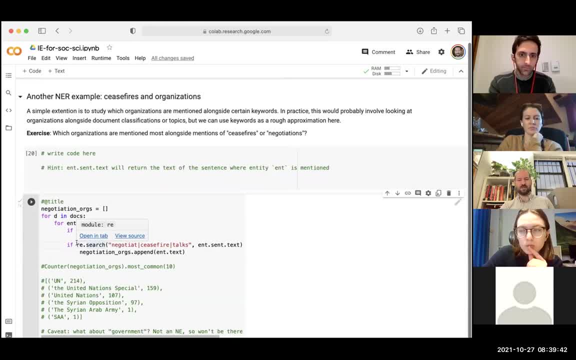 a word. we can check to see if a lemma is in a document, but in this case, since we're just doing it quick and easy, We can search for some of these terms like negotiation or ceasefire talks In the sentence that that that entity is in. 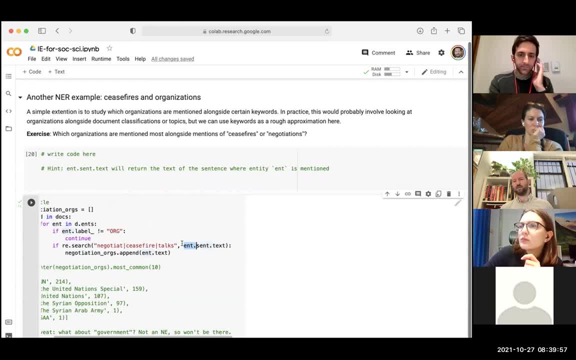 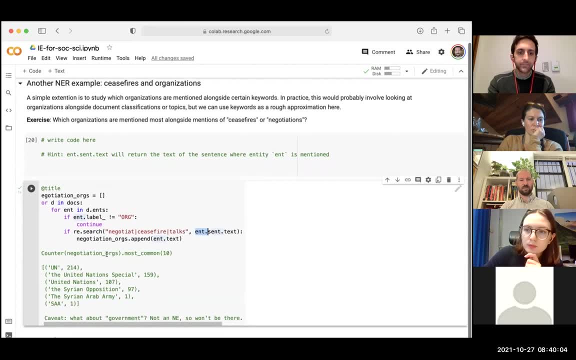 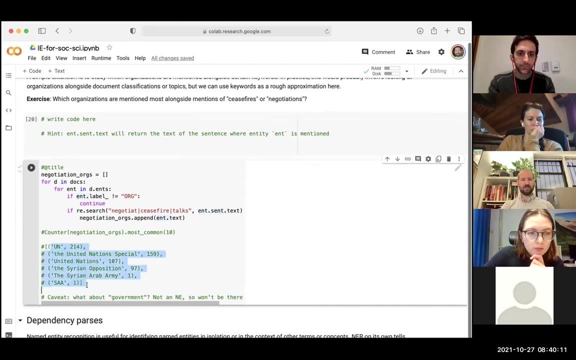 Right, So we can also this at the document level, or look at a window of words around it, And if we, if we find those terms, add it to our, our list. And so if we do the same counter thing, we see something that makes a lot of sense, which. 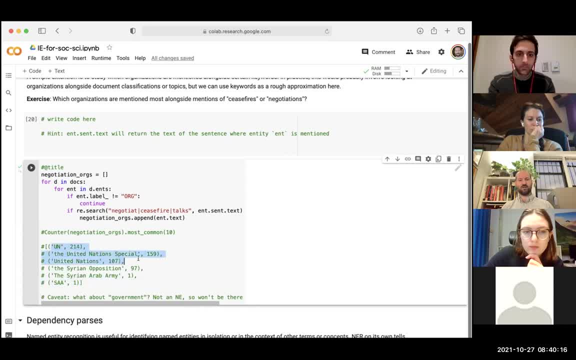 is a lot of the organizations that are mentioned. alongside negotiations or ceasefires are the UN or the UN Special Representative to the Syrian conflict, And so again, sort of. I think it's always important to think about the both the biases in the model, but also the biases or the limitations of the tool that we're using. 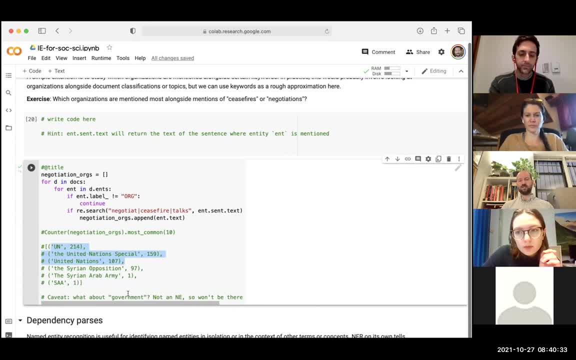 And in this case, you know, if you imagine, a typical sentence might say: the UN is brokering a ceasefire between government forces and the Syrian opposition government is not a named entity, so we, we might systematically undercount things like mentions of the government. 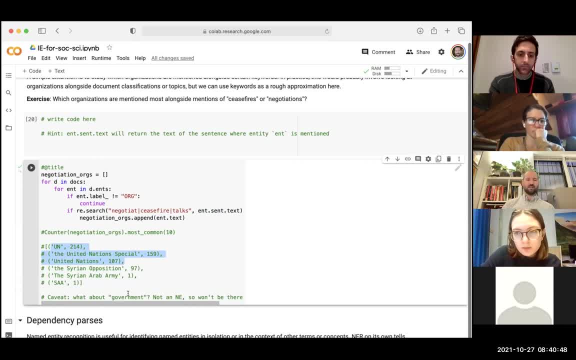 precisely because it's not a name yet, Right? So I think It's always important to think about the limitation of the model, but also the limitation of the sort of the conceptual approach that we're using here. Okay, other other questions on named entities? 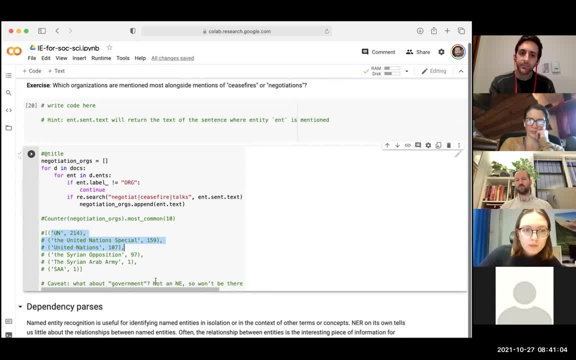 Before we move on to dependency parses and some some rule based extraction methods, Feel free to drop in the chat and week. oh, Andre, yeah, yeah, I have a maybe a bit more specific question. So I'm working on a project that involves articles or events with kind of continuous 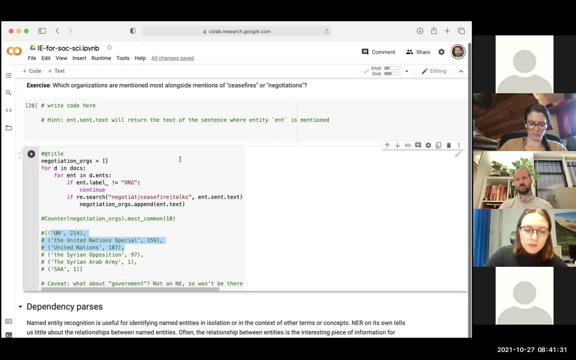 coverage to some event, may have, let's say, multiple articles referencing it. And, and I was wondering, is there a way to kind of combine clustering with named entities? you know, so I'm trying to kind of just use generic kind of clustering algorithms to combine. 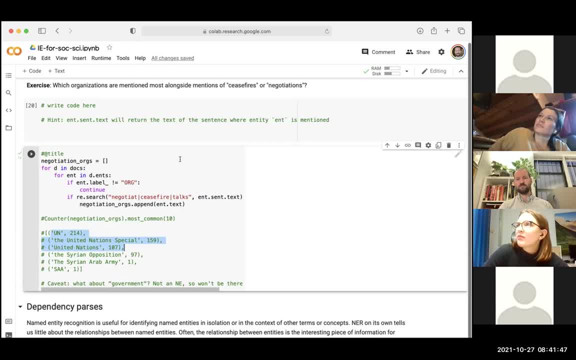 these articles together. But I was curious if there's a way to kind of cluster On On the name entities or something like that. Yeah, so so that especially the sort of event disambiguation or sort of duplicate event detection is is really hard and not not solved yet. 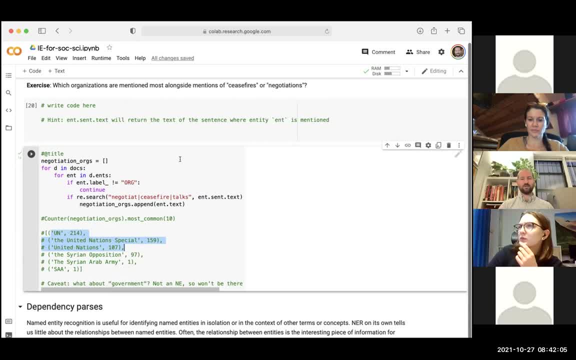 I think, I think in that I think more specifically for what you're describing, probably the way to do it is this sort of entity lookup or entity resolution step I was talking about earlier, where we're basically the sort of conceptual framework is for every. 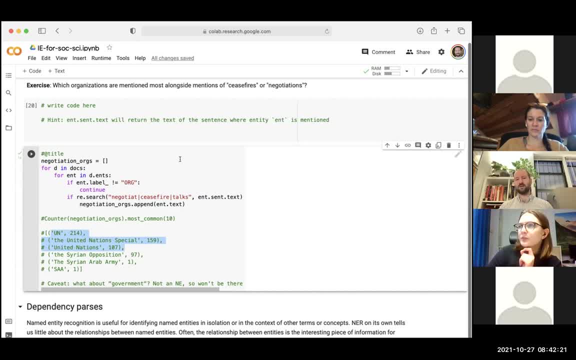 mention of an entity. Can you figure out the Wikipedia article for that that entity? right? So the UN and the United Nations both have the same Wikipedia article, And so we're just trying to resolve different mentions to the same entity identifier as a way of essentially doing clustering, but sort of in a sort of lookup sense. I had some. 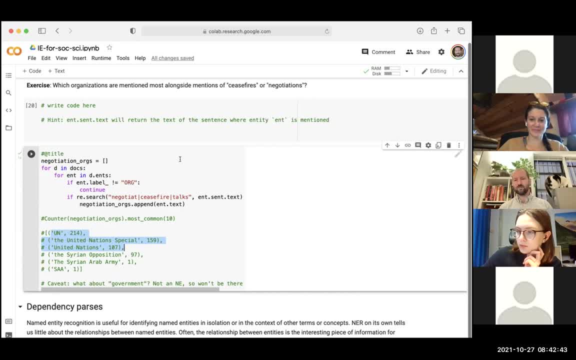 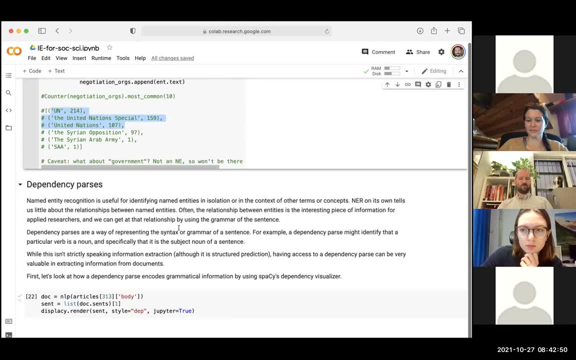 other things I can, I can recommend. if you send me an email, I can, I can send them to you. Okay, We're good. Okay, I want to move on to dependency parses, because I want to make sure that we have enough. 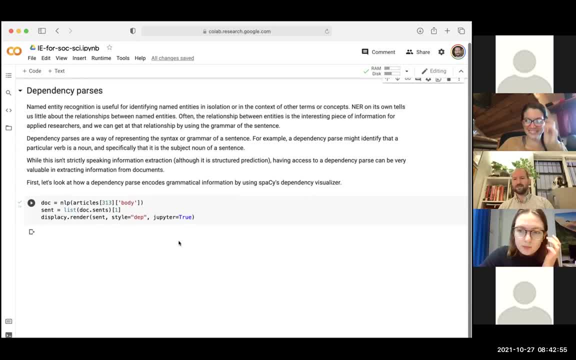 time and I have to, unfortunately, leave right at 11 to go see Katie and Ian, So okay. so named entity recognition is useful for identifying named entities, obviously, but it does so in in isolation or in the context of mentions of terms or concepts like 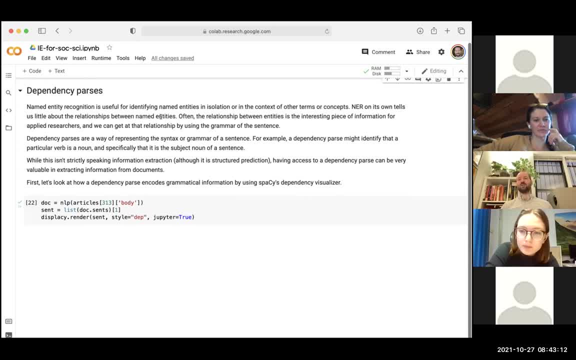 we just did before, So it doesn't give us a lot of information about the relationship between entities and the social scientists. That's, that's often sort of the core of what we're interested in. Okay, So what's the first thing that we're interested in, which is: how do political actors interact? 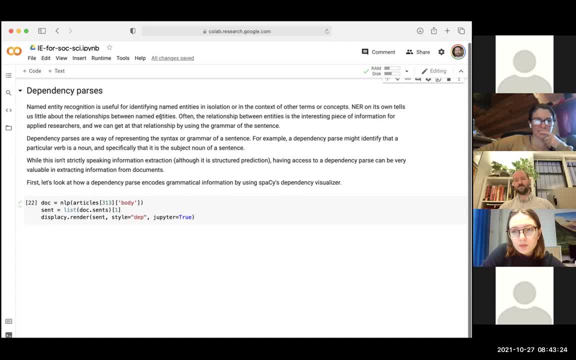 with each other? What? what behaviors are they undertaking? What's the? what are the bureaucratic or organizational structures that bind them together? And one way of getting at that is by using the grammar of the sentence. So dependency parses are a way of representing the syntax or sort of think of it as grammar. 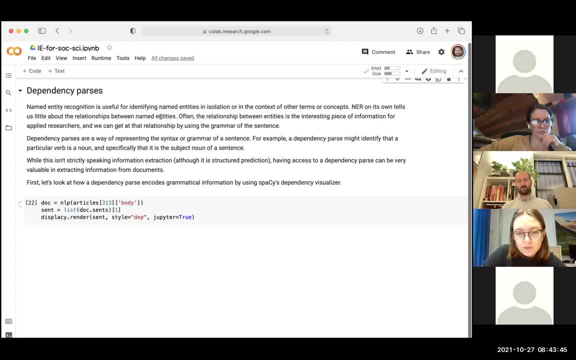 of the sentence, And so if you've come across something like part of speech tagging or language tagging, or or learn this in a language class, you get used to saying, okay, this word is a noun, or this word is an adjective, or this word is is another noun. 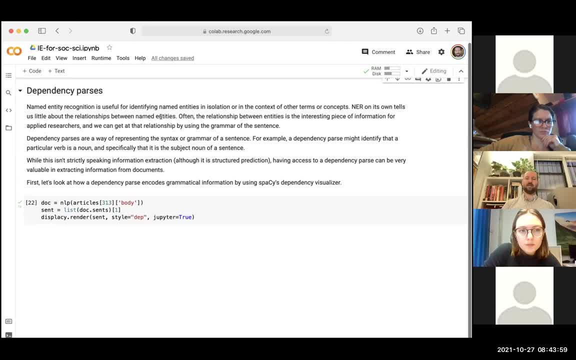 And what dependency parsing is is essentially a layer on top of that- that say: not only is this adjective, this word, an adjective, it's specifically an adjective that modifies this noun. or not only is this, a, this, this word, a noun, it's specifically the direct. 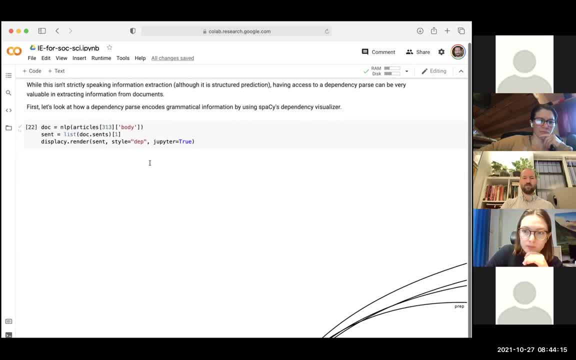 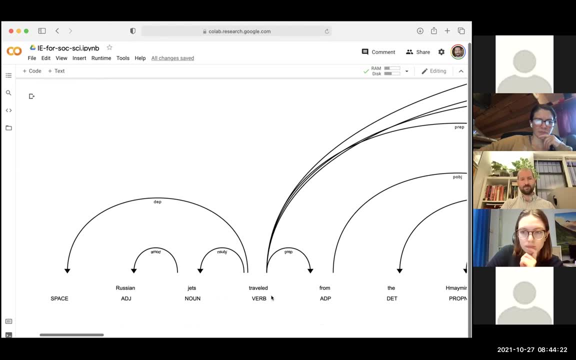 object that belongs to this verb, And so a nice way of visualizing this Is as a, as a directed graph, right? So we have something like a, like a verb here and then a noun, and this noun is specifically the subject noun of this verb. 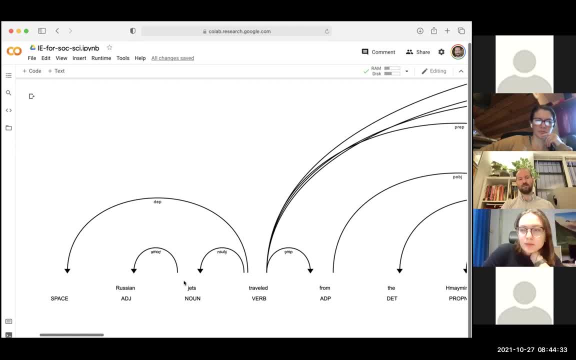 And this word is an adjective and it's specifically an adjectival modifier of this word, And so it's. you think about it as sort of a layer on top of a part of speech, tagging down here. that gives us the relationship between words. 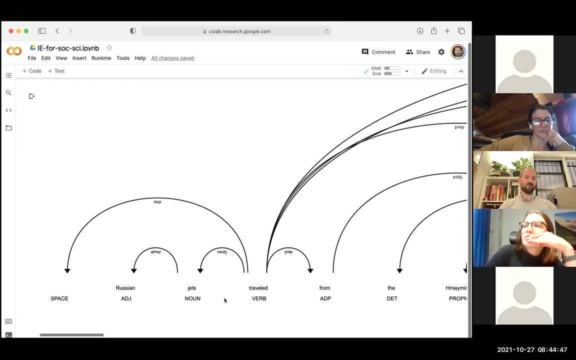 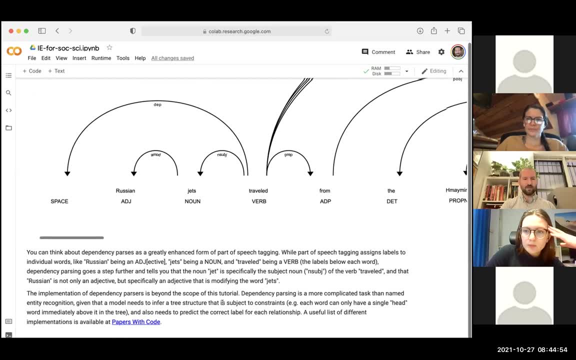 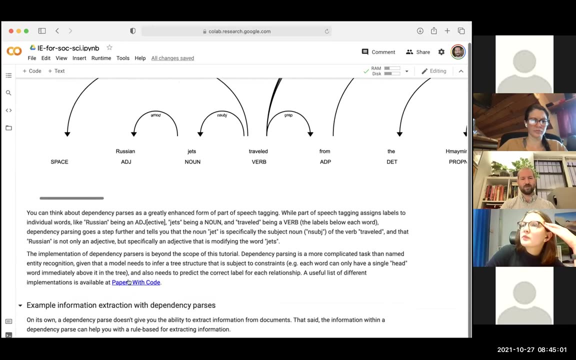 And and this is a way that this Let's us extract the relationship between entities in a way that I think can be quite powerful and relatively easy to do. So I'm not going to get into the details of how this is done. You can look up a large collection of papers about how it's done right here. 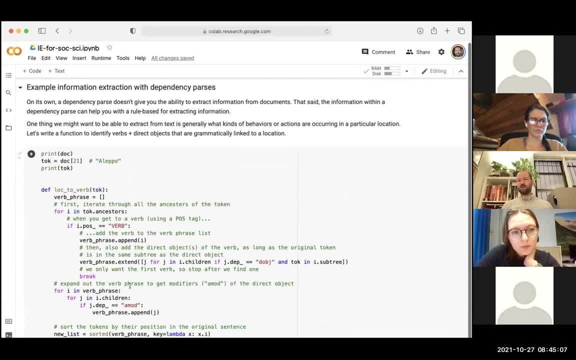 Okay, so so dependency parsing on its own is not a form of information extraction, right? It's sort of a way of marking up tokens with extra information about how they relate to each other, But that information gives us ways of of writing rule based systems for for extracting information. 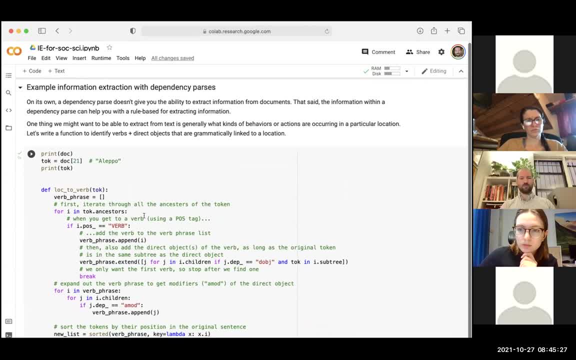 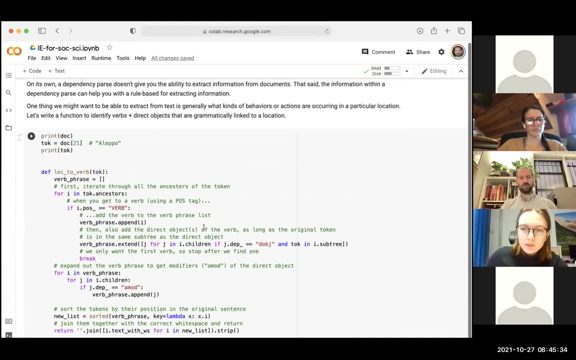 from documents. So I'm just going to walk through what's going on here, which I think is is a little bit confusing when you see it for the first time, But if you just scroll back and forth a lot between this and the and that sort of arrow, 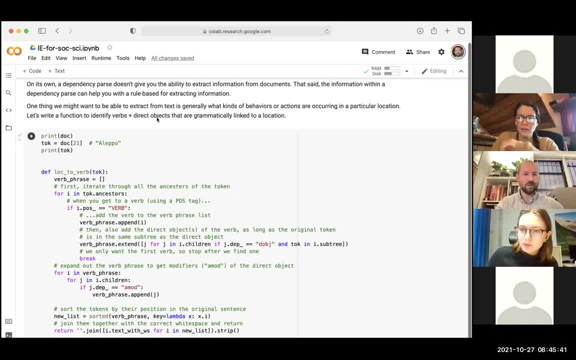 diagram above, I think we'll start to make more sense. So so one thing that we might want to do is, you know, we're going to go back and forth. we're going to go back and forth a lot between this and the and that sort of arrow diagram. above, I think, will start to make more sense. So so one thing that we might want to do is, you know, we're going to go back and forth. we're going to go back and forth a lot between this and the and that sort of arrow diagram. 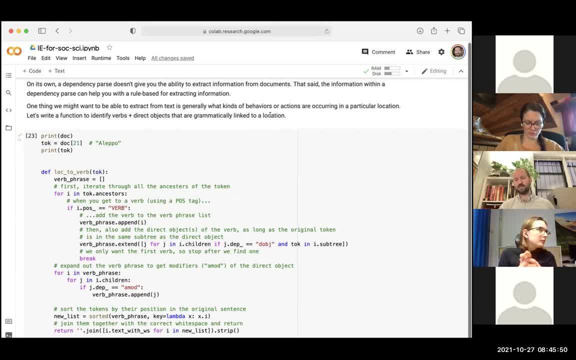 above. I think we'll start to make more sense. So so one thing that we might want to do is, you know, we've identified a lot of locations in our, in our, in our corpus of text. we might want to have some sense of what's going. 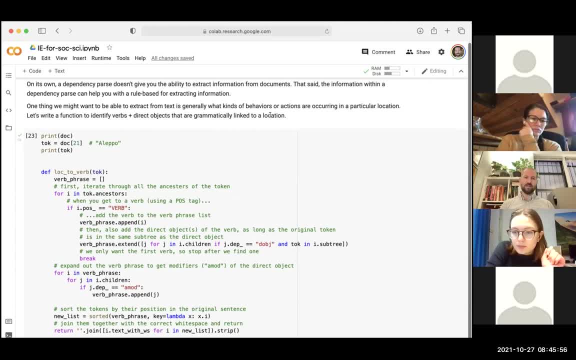 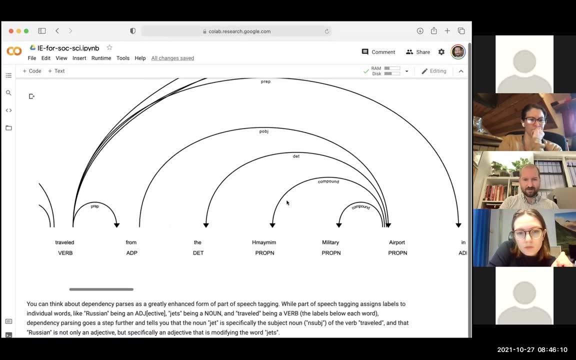 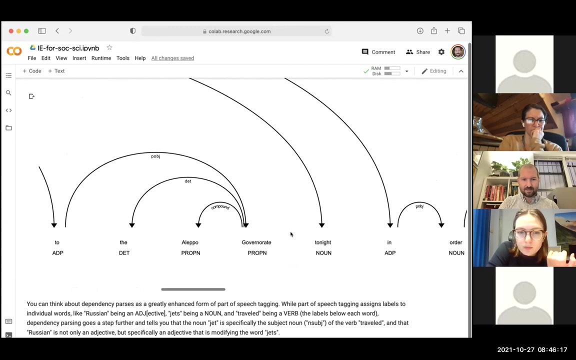 on in each of these, these locations, And so one way of specifically operationalizing what's going on is what verbs and direct objects are grammatically linked to this location in text. So we scroll back up here: Here's the location. Yeah, okay, so here's the location, and we might want to figure out, okay, what, what? 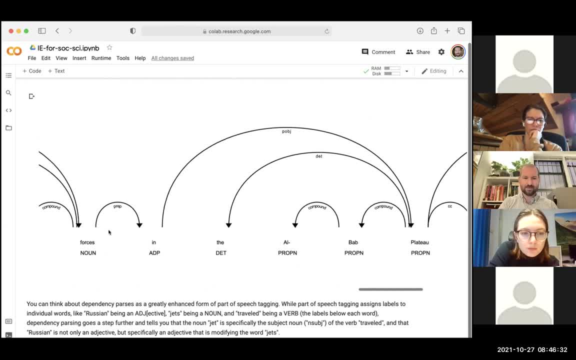 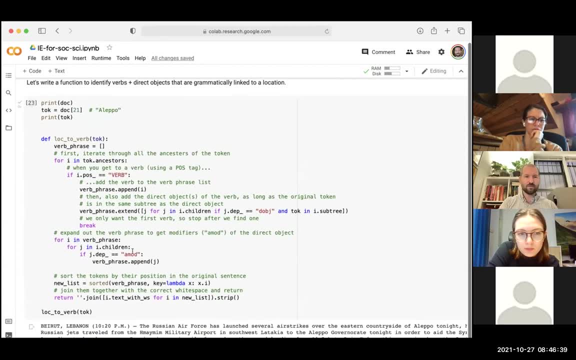 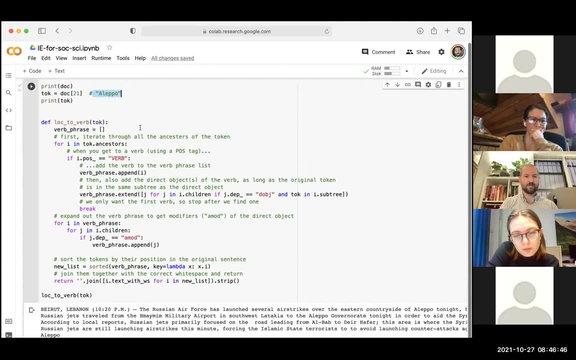 verb and direct verb is happening here right, so we can keep sort of moving up the tree until we get to battling, for instance. So we're going to do this by looking at the Aleppo, the mention of Aleppo in the document above. 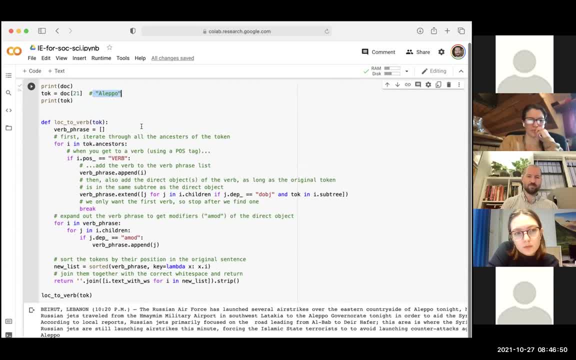 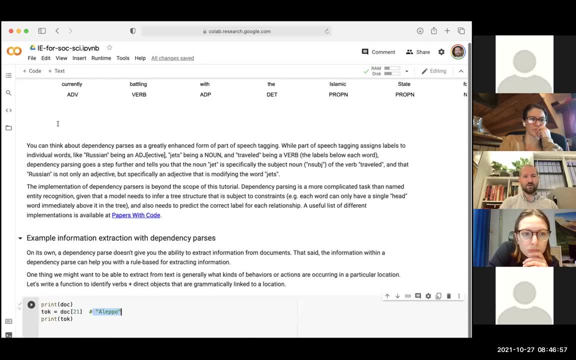 And I'm just gonna walk through what the code is doing and then stop and sort of check and make sure that we're all. we're all set here, Okay, so you know, this is a, this is a directed graph here. 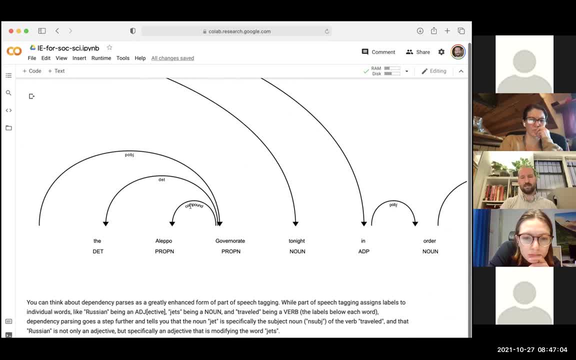 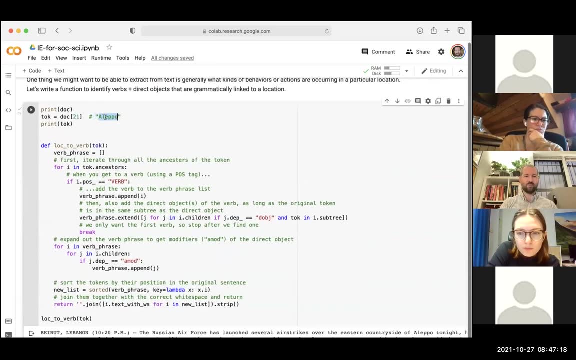 And so we can think about moving up and down in the dependency tree, right, so? so moving up is going backwards with the arrows and then going down is following the arrows in their, in their direction. Okay, All right. So if we have a word Aleppo and we're trying to figure out what verb is, sort of grammatically, 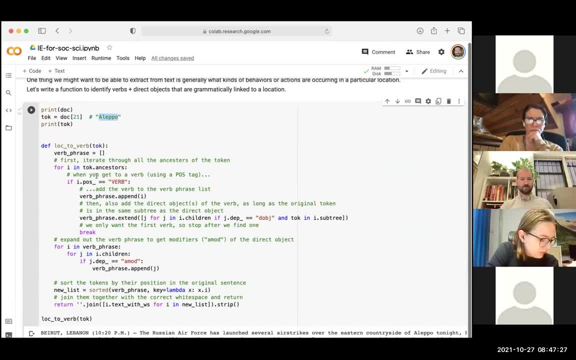 what verb makes most sense is sort of the verb that's happening in that location. One way we can do that is by saying, okay, let's, let's go up the tree right to look at the tokens that are above Aleppo. 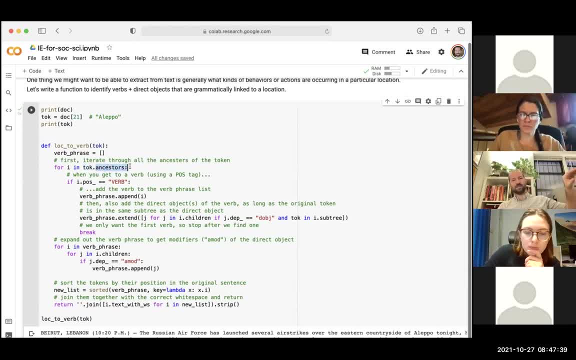 So, following the arrows backwards, we can get with this ancestors attribute And we're going to keep going through those ancestors, Okay, And then we can add that to a word, that's. that's a verb, right? So here we're using a part of speech tag. 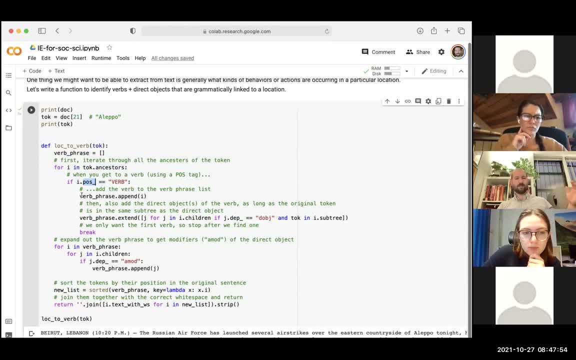 So go up until we find a verb and add that to our sort of list of verbs. Then you know we, we don't just want the verb on its own, because it might be things like launch, and we don't really. we want to know what's being launched. 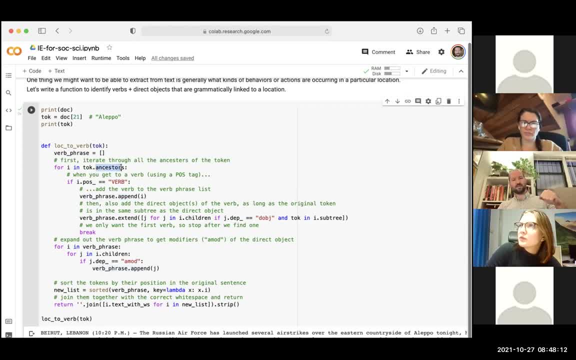 So then we can not not go up to the ancestors, but instead look down the children of that. It's a. the children are all the, all the things below it in the, in the arrow, and look for words that are a direct object, right? 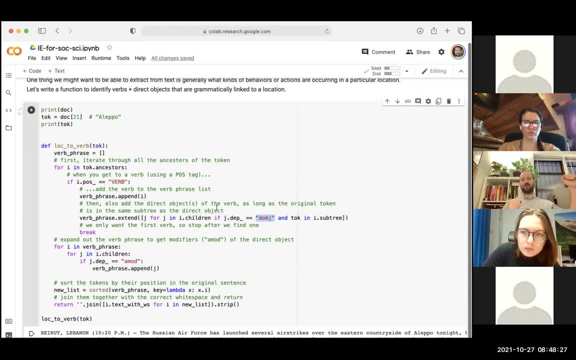 So we've started with the location, We've moved up to find a verb, and then from the verb we've moved back down to find a direct object and sort of for our oh yeah, So the verb, the direct object, but then we might also want any of the adjectives, right. 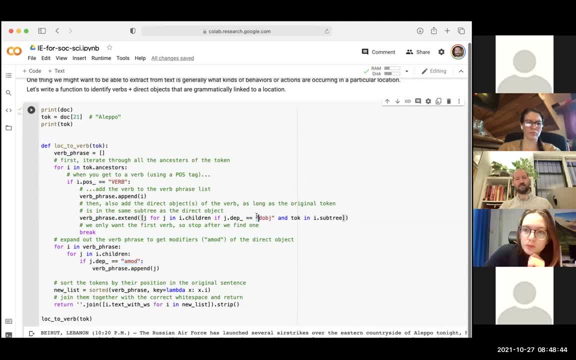 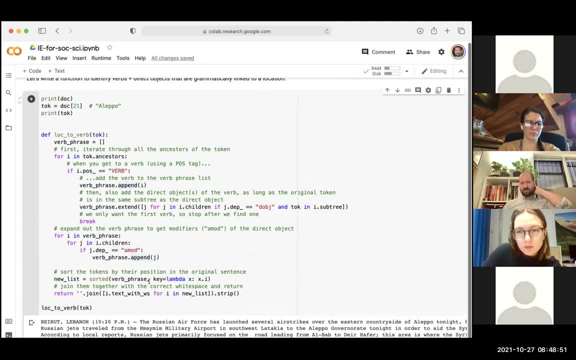 So we can go through and see: is there a, is there an adjective? Okay, So we can go through and see: is there an adjective that modifies this direct object? And if there is added to the verb phrase, right, So we've. what we've done is we've said a way of operationalizing what's going on in. 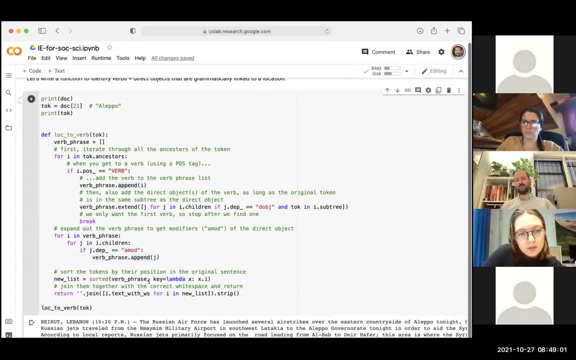 a location is to look at at sort of the parent verb and any direct object that's a child of that, of that verb for that location, right. So we move up, we find the verb and we move down and find the direct object that's underneath. 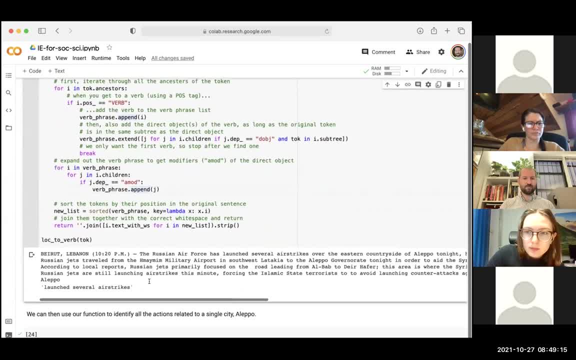 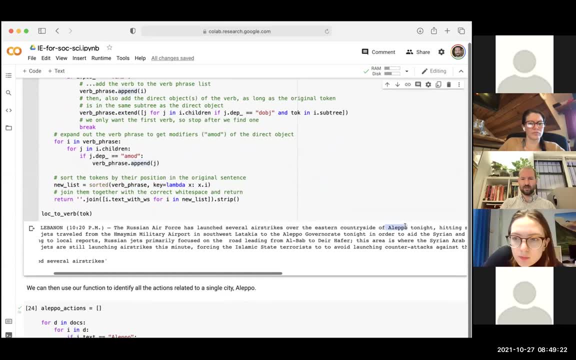 it. So if we, if we um apply this function to this, to this document, um, so here we have Aleppo, um, it's going to move up to launch and then take airstrikes as the direct object and several as a modifier and give us, uh, launch, several airstrikes. 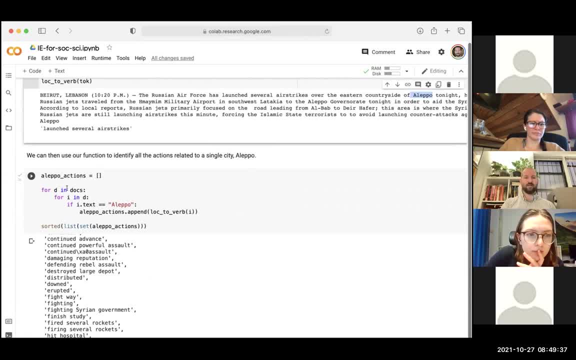 Okay. So what this looks like. if we apply it, um once again, to all the documents in our corpus, we can say: um, go through each, each document, Okay, Okay. So if we go through each token in the document, if that token is Aleppo, apply this function. 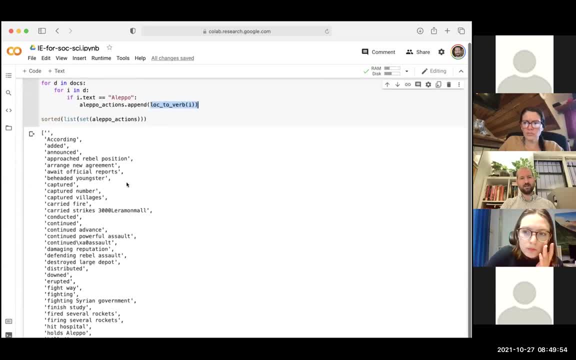 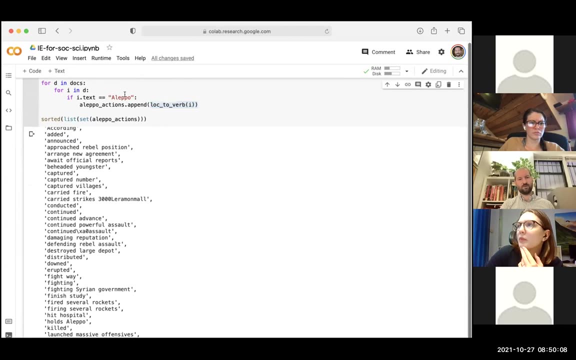 All right, And so then we get out sort of a list of different things that we could sort of call events or actions or behaviors that are occurring in this location, Right? So, um, this I think, if if you don't know a lot about what's going on in Aleppo, this 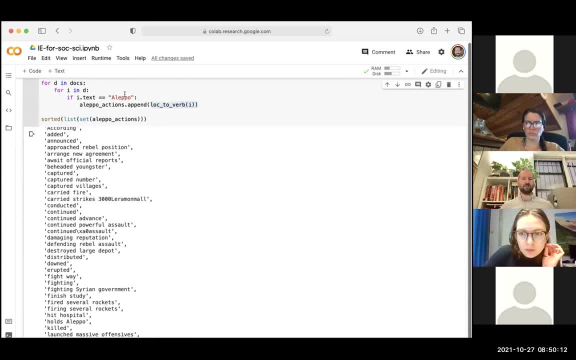 is a way of giving you sort of some immediate context of um, what kinds of actions are happening here, Right And so, as we might expect, there's a lot of um, especially in this period. there's a lot of fighting in Aleppo. 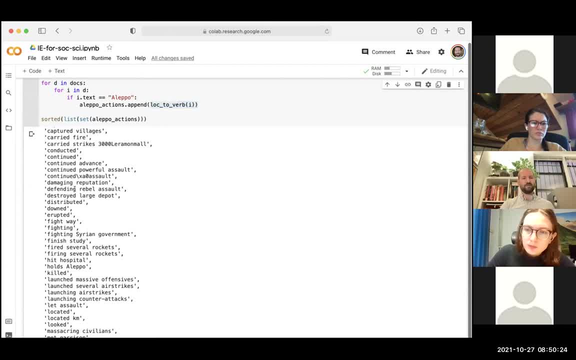 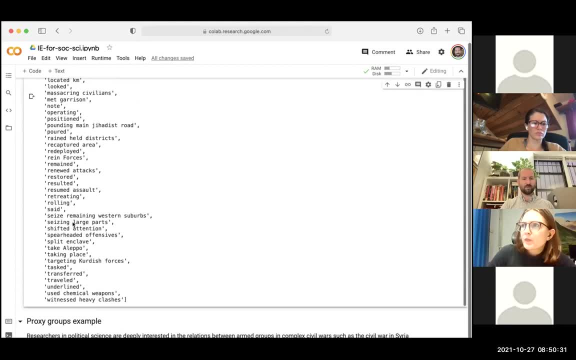 So there are. there are a lot of um sort of defendings or beginning attacks or launching offenses, or launching airstrikes or destroying um property or killing people, Um so this: this is a way of pretty quickly getting a sense of what's going on in this. 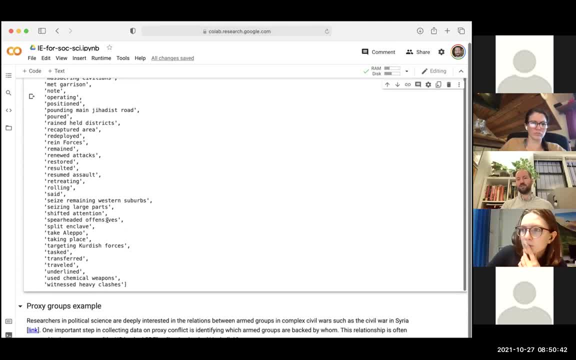 location And I think, once again with, as with most of the examples here, this is pretty descriptive. It's not. It's not going to sort of give us the answer that we're going to put in our social science paper, but you can imagine how you could, you could extend this and say, well, we don't. 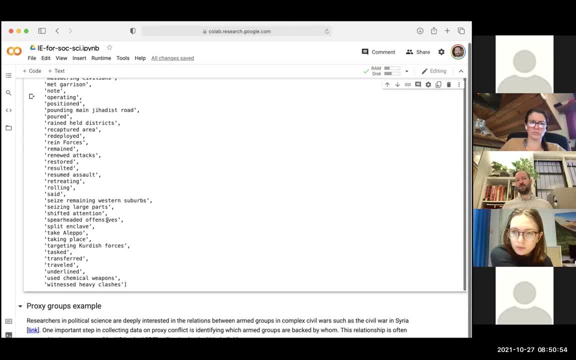 just care about Aleppo. We care about um, all of the locations, and we also care about things over time. So if we wanted to answer um, for instance, how, how has, how has the use of airstrikes changed over the course of the conflict? or changed geographically over the course of? 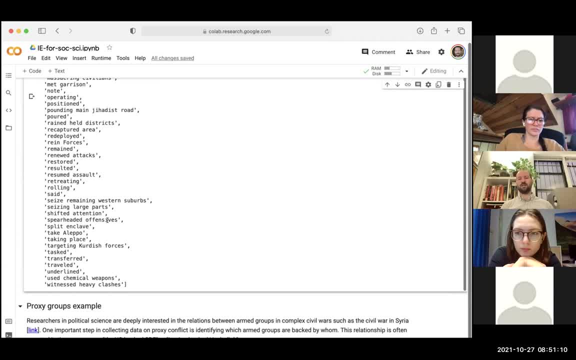 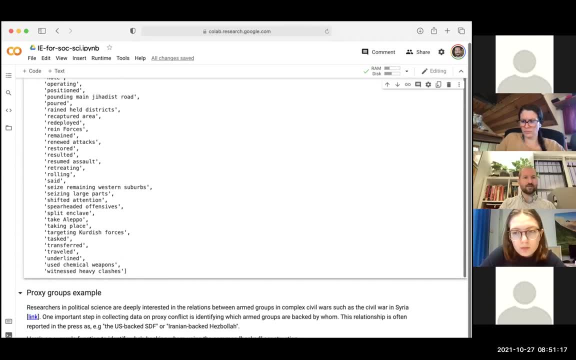 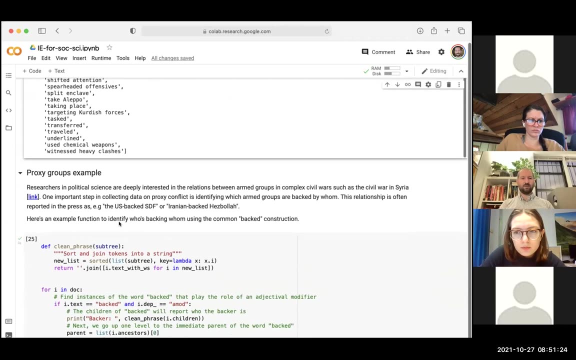 the conflict. this is a way of starting to extract that information that we can then use downstream to answer our question. Um, I see something in the link, uh, so there's another example here, uh, looking at at proxy groups that I think I'm going to skip, but you can go back and and um, look for. so. 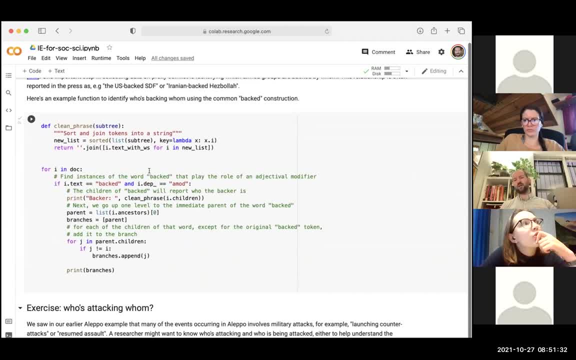 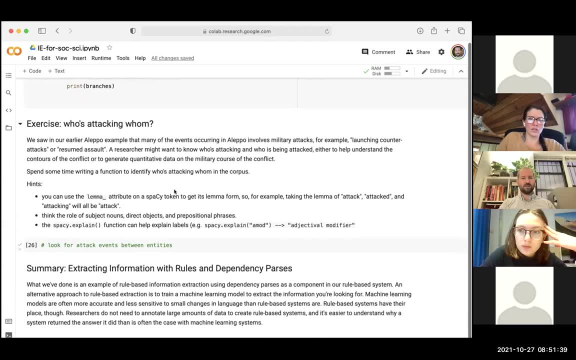 just just another example of how you can use these tricks of moving up and down on the dependency tree to to get the information that you're interested in. uh, there's, there's one other exercise, uh, that I wanted Um to give you, um to sort of get a sense of of going back to more of the named entity. 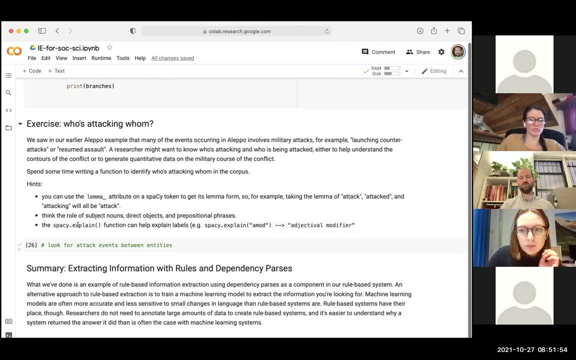 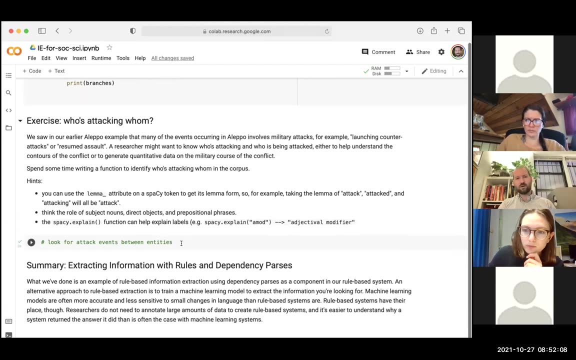 stuff. So, um getting a sense of who's attacking whom or when, when these military offenses are happening, who's the person, who's who's um instigating them and who are they being instigated against? Um, we are, I don't know. 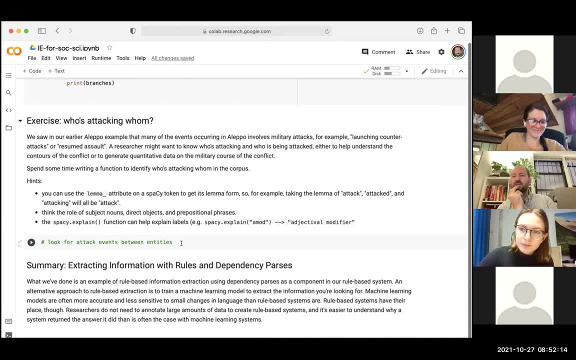 Okay, Um, I guess I'll. I'll appeal to the organizers here, Is it? is it more? do you think it's more useful to go through this exercise now or finish up with the prepared stuff and leave this as a as an exercise for the reader? 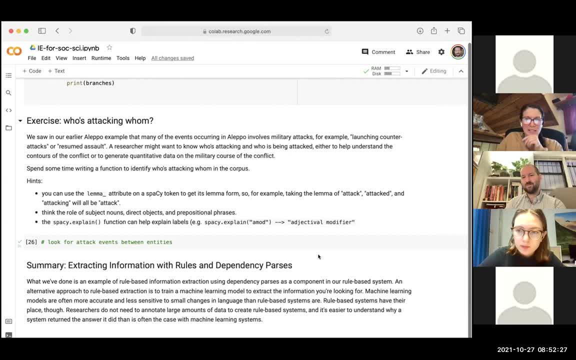 Yeah, we have about eight minutes left, so maybe you talking especially for our non-live participants would be best. Um, and then folks can use this notebook for as long as they want. um, essentially, Yeah, No, I'm happy to email about it too, or or chat. 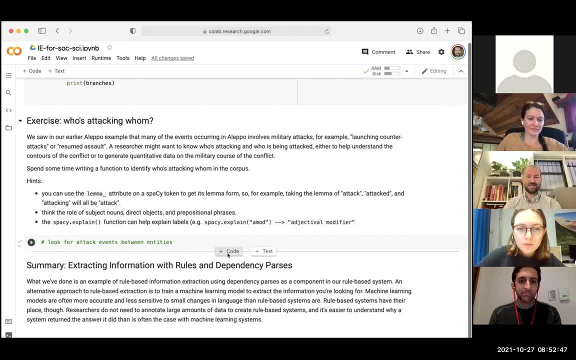 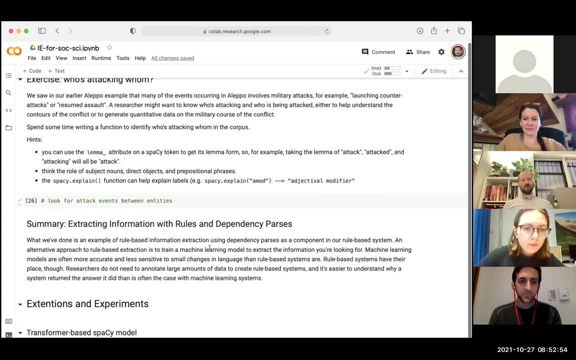 Um, see what you see what you come up with. Uh, this one that is actually not code, because it's. I think there are a bunch of different ways of doing that, Okay. So just just to summarize, sort of this, this section here, uh, dependency parses themselves. 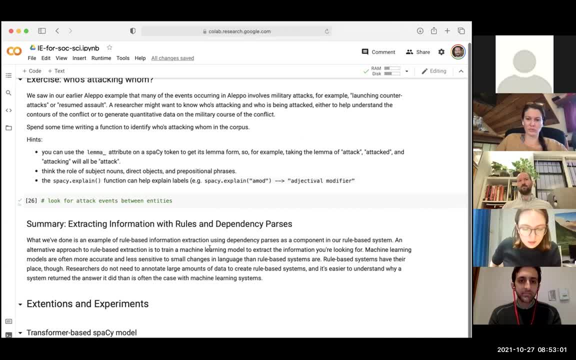 aren't information extraction, It's. it's a way of basically marking up a document with more information about the grammar or structure of the document, but we can use that, that information, along with rules, to extract pieces of information we care about. Okay. 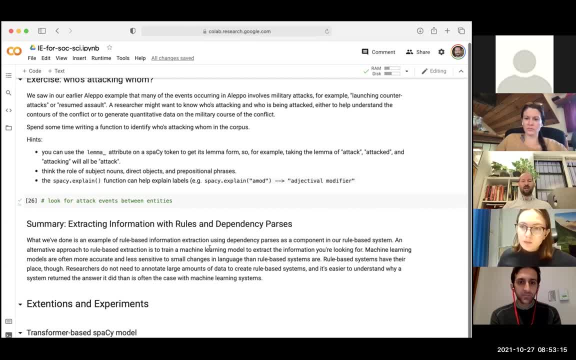 Uh, one caveat is that, in terms of accuracy um and robustness to to the intricacies of language, this, this rule-based approach is- is probably not the most accurate way to to extract things like what we just extracted above. 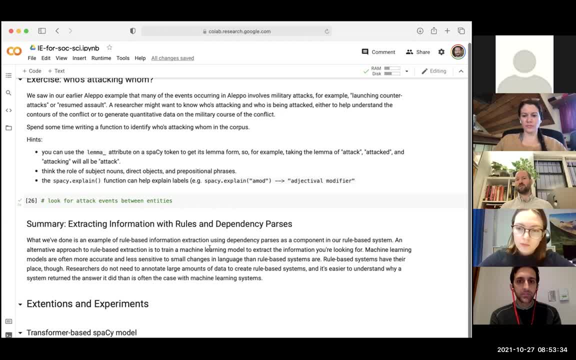 And so, there, there are a lot of different ways of expressing something, And if, if our rules are are off, we're going to, we're going to miss certain ways of describing an event. Um, on the other hand, Okay, 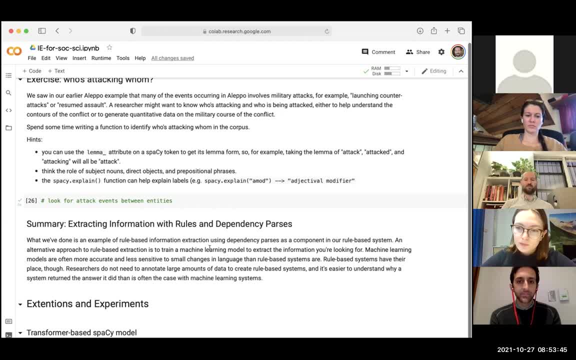 This. this approach has a lot of benefits compared to uh, sort of machine learning based approach. Uh, first of which is that, you know, it took me maybe 10 minutes to write that extractor above, which is much, much faster than annotating potentially hundreds or a thousand documents. 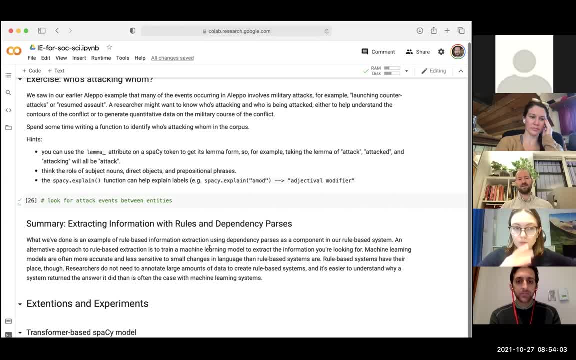 figuring out the architecture of a model, training and tweaking it, deploying it, Um, so for, for tasks where sort of speed is is important, um, or if you're doing exploratory research, Okay, this kind of technique is really helpful. 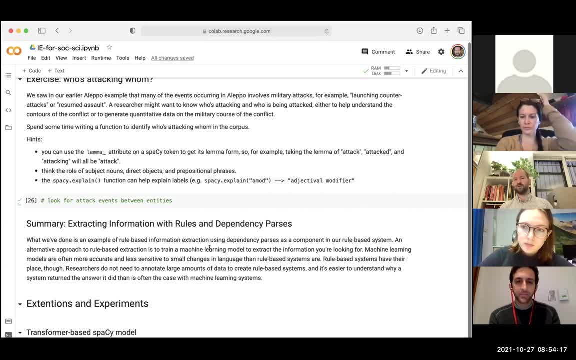 Secondly, it's also very easy to explain what's going on here So you can put in your paper: you know, we identified, we identified place names this way and here's how we extracted um sort of what we're calling an event by using this. 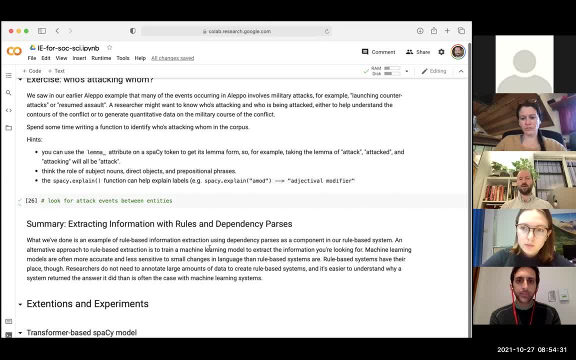 dependency tree, Right, So you can put it in the paper and it's very clear what's going on. and it's often more difficult to explain, uh, the outputs of a of a fully machine learning based approach. Um, okay, Great. 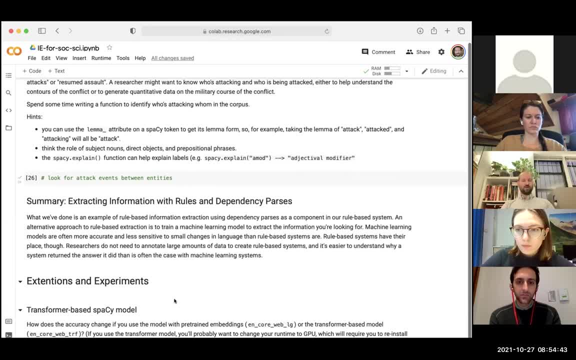 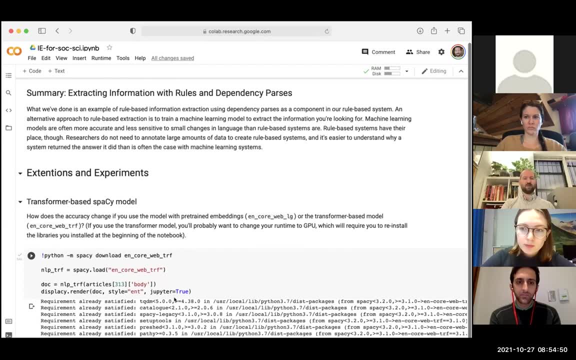 Thank you, Okay, So then, uh, I just wanted to walk through some stuff at the end of the notebook. Um, I don't think we'll we'll run all of these, but I wanted to bring them to your attention because I think. I think they're interesting. 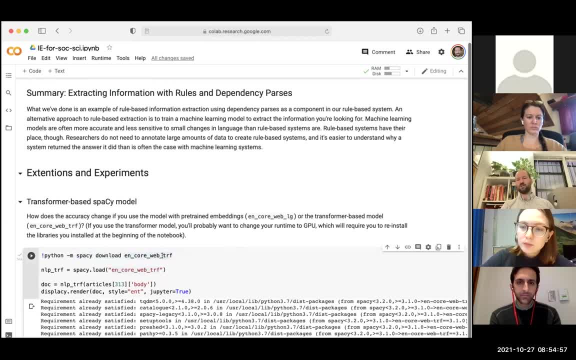 So one of them is is spaCy has a another model that's. that's larger and transformer based. So I mentioned earlier that, um, the models we were using before were um used convolutional neural networks. Um, this model uses transformers and is is noticeably more accurate. 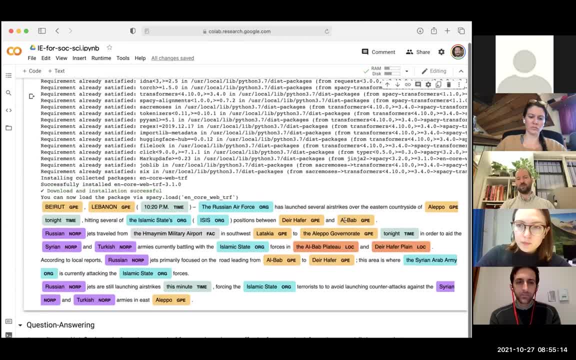 And so if you, If you download it and and apply it to the same document we looked at before, it starts to get things better right. So these locations were wrong and it now gets them correct. The Islamic state issue is, um, still sort of more of a social science issue, I think. 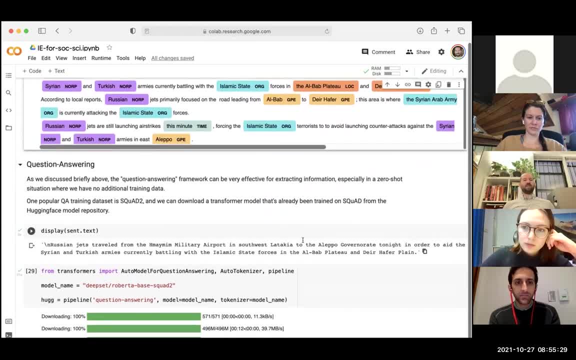 than a machine learning issue. I also wanted to mention, very briefly at the end, um, a different paradigm to information extraction, called question answering Right. So, um, this is something that that Katie and I worked on in a, in a paper, and then. 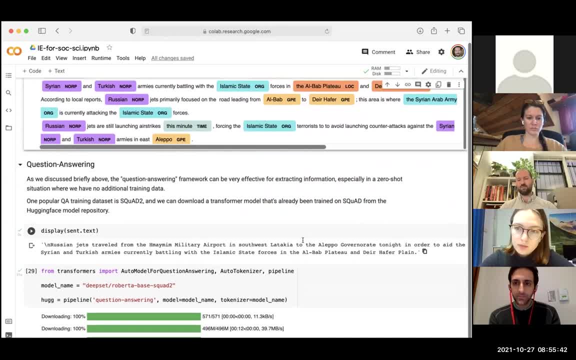 we found, Um it was. it's a piece of the same piece, Um, I also think it's so similar to, to the, to the, to the. uh, how, these two different pieces? Yeah, I guess I can say it's, it's more. I mean, I came up with this, I guess I believe. but the thing is, I think, the, the, the important thing is when the, what we do is we, we deal with the, um, you know, like the, the, the, the, like the, uh, the, uh, the, you know. the theory of, of the, of the theory of, of the theory of the problems we have is that we try to we, I was, we as, as a uh, a, a later on, I, uh, I try to identify the. 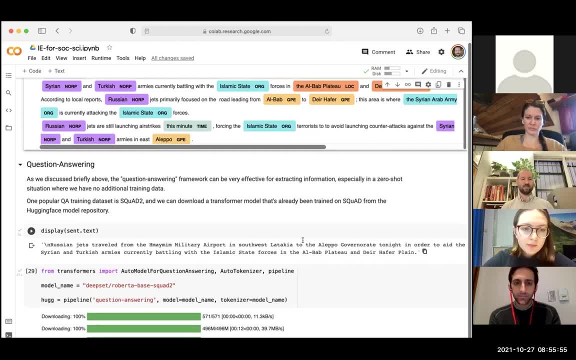 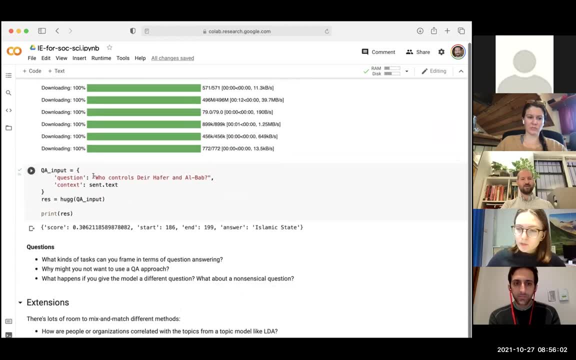 problems, the problems of the, the problems of the information, with that, um, that protest and essentially the. the framework here is is really, uh, quite simple. you know, you give it a piece of text and a natural language question, so you, you write sort of a. 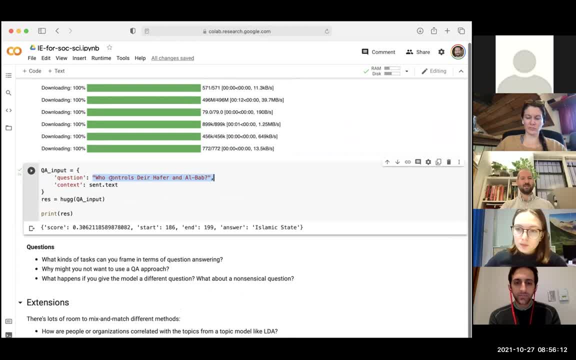 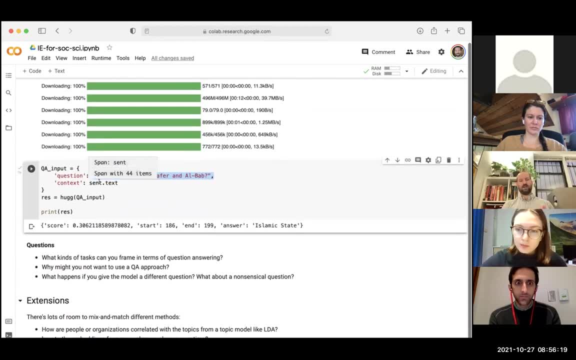 question in a way that you would ask a person um something like: who controls der hofer and all bob um given the sentence and the model will return um the the span of of text that it thinks answers your question right. so either think about this as um as extractive question, answering you give. 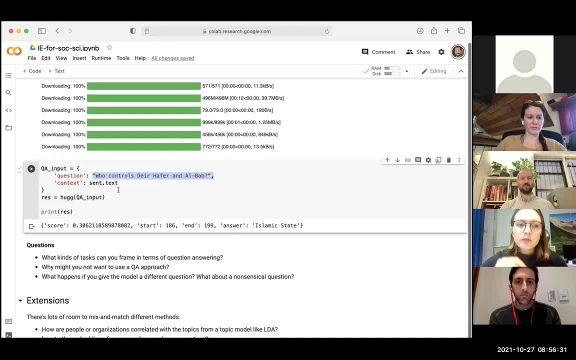 it a question and it it returns a passage of text that i think thinks, uh, best answers your question, right? so i think these have gotten um, these models have gotten a lot better recently, um, and i think they have a lot of. they all have a lot of applicability because they don't require. 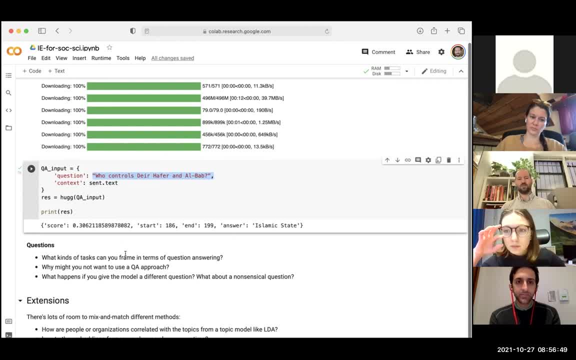 in some cases, additional training data right. so there was no like tweaking this model on my question, like this specific who controls question, or fine tuning it on the specific text. it just works. um, i would encourage you to put in some other questions here, um, including questions that don't make any sense. 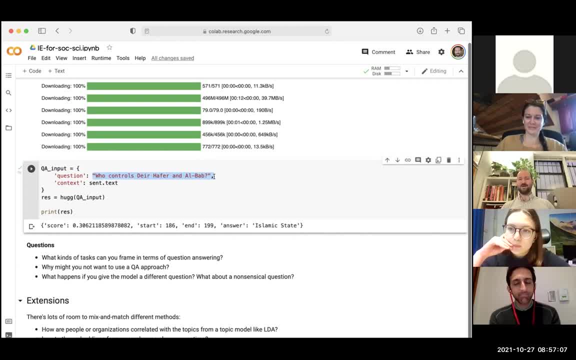 and you'll quickly see that you get answers that don't make any sense, right? so these, these models, i think, are exciting because in some cases they don't need any additional data, but there are also a lot of pitfalls, in that they will often fail in ways that are. 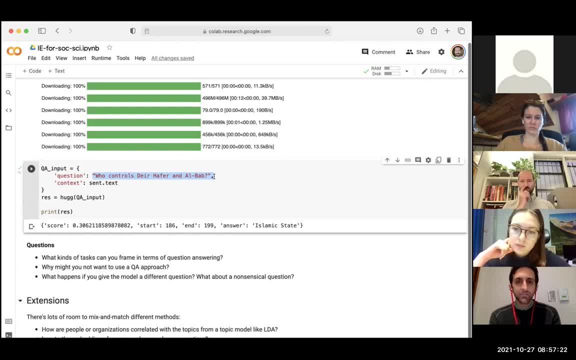 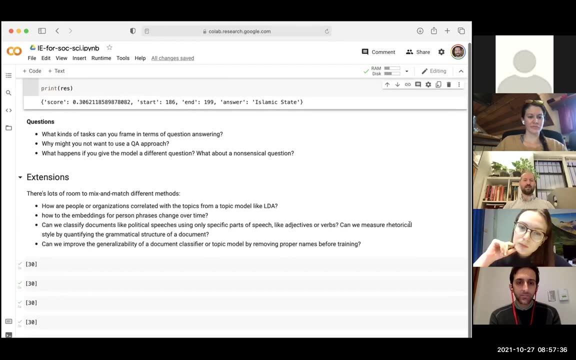 are non-obvious, so they'll give you an answer, oftentimes even if it's wrong. right, so i think it's. yeah, i would encourage people to think about situations where question answering works, in situations where it might not work, and then, finally, at the end, i wanted to bring up some, some extensions or ways of thinking about this. 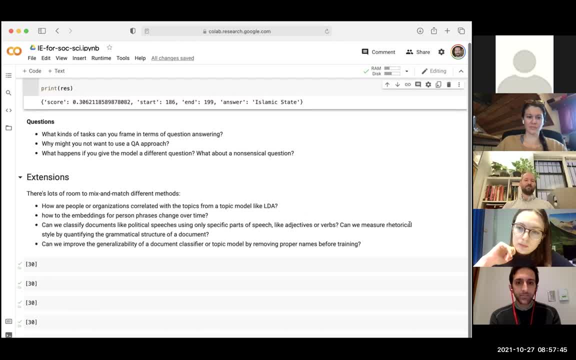 in your, your own research, and i think that information extraction techniques become really powerful when they're used in conjunction with each other- the two different techniques or in conjunction with another technique, right? so, um, so, if here's a sort of a list of illustrative questions, like you know, you can run. 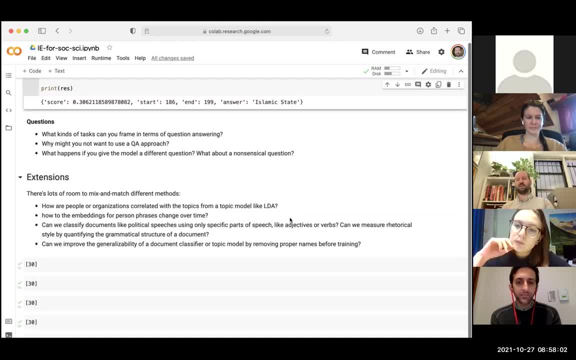 a topic model and then do named entity recognition at the same time and answer questions like which organizations are mentioned alongside which topics? right, which is a lot more interesting than here are the topics or here are the named entities, or um, you know, i uh, i think con someone. yeah, connor. 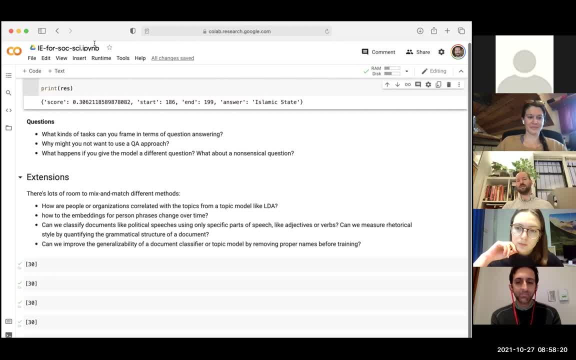 mentioned earlier about discovering n-grams. you could use named entity recognition to discover n-grams. um, and say you know this whole, this whole name is one token- and then learn an embedding, or learn a dynamic embedding and see how that sort of changes over time, what the embedding looks like. 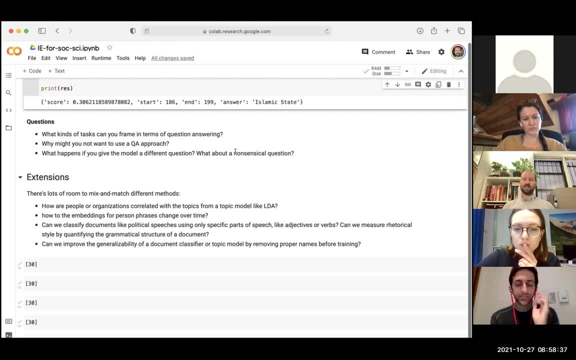 over time. i think there are other things like: can we classify um speakers, uh, political affiliation by looking at just the grammatical structure of their, their sentence? or can we look at just the adjectives that people use as a way of classifying their, their identity? or um, their partisan identity?